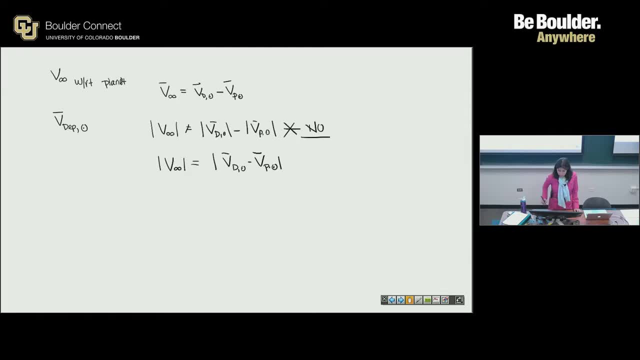 we don't want to do. You want to take the magnitude of the difference of the vectors. that way you're accounting for the direction of the velocity and not just the speed. okay, The second thing is on the homework with Vesta and Ceres. 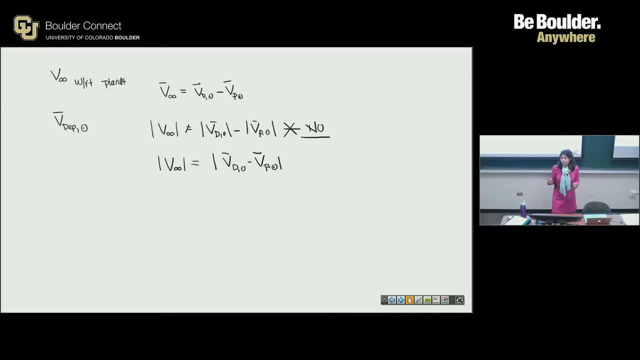 when I gave three assumptions. you're not solving the problem three different times. okay, It's not part A, B and C. Some very enthusiastic people wanted to solve it three different times. It's just, you just solve it once with those three. 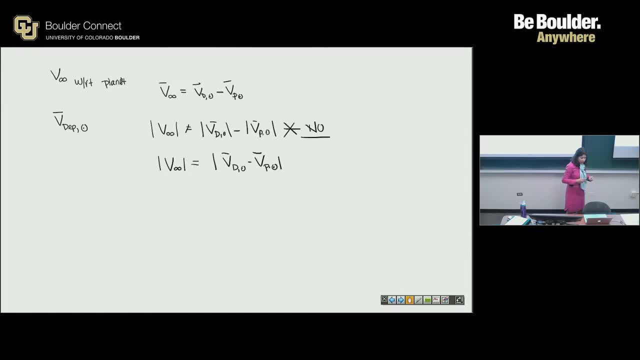 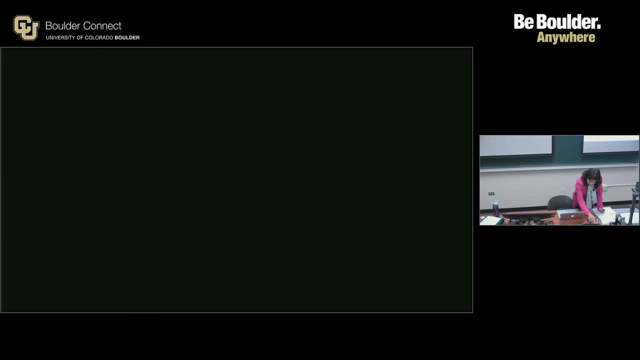 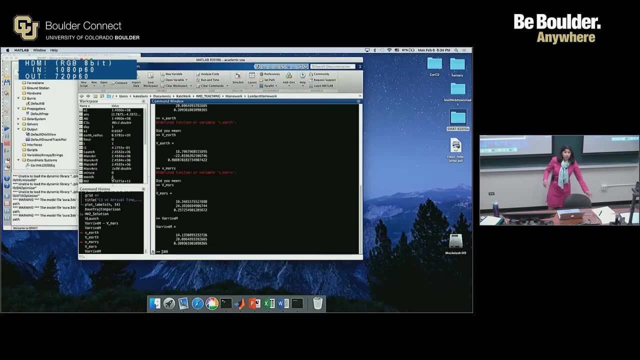 assumptions. And then let me see what other things were we having. Let's see here: Does that pull up my laptop? No, it did not. Okay, here you go. One issue that I'm going to try and replicate this here in GMAT and this: 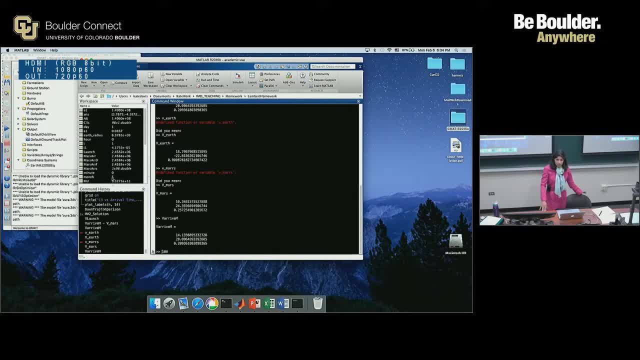 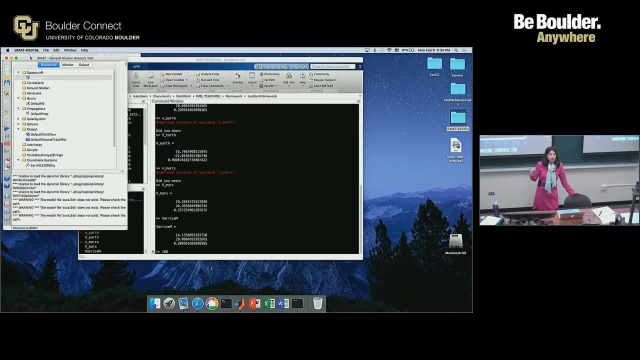 might not be a bug in Windows or on the computer, It might only be on the Mac. GMAT sometimes has the annoying way of not applying corrections that you think they are, and this is especially the case with copy-paste, And I know that when there's. 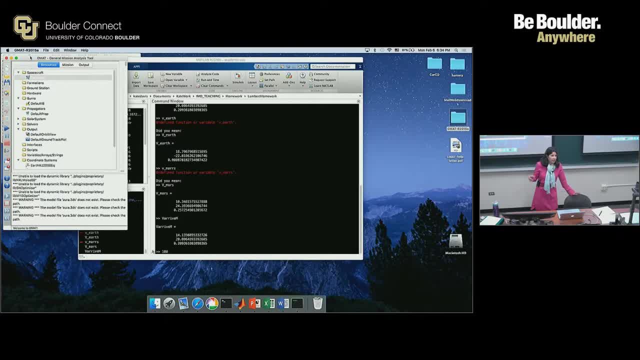 really long sequences of numbers, especially like when we give the semi-major axis and the eccentricity, it's really common to want to just copy-paste. I'm going to see if this works okay. So let's say I want to try and change my. I'm sorry that's so small, my x. 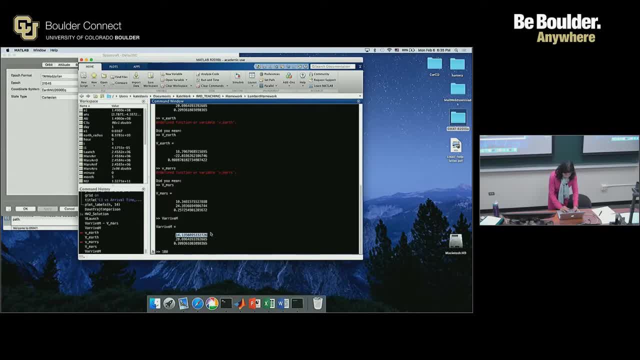 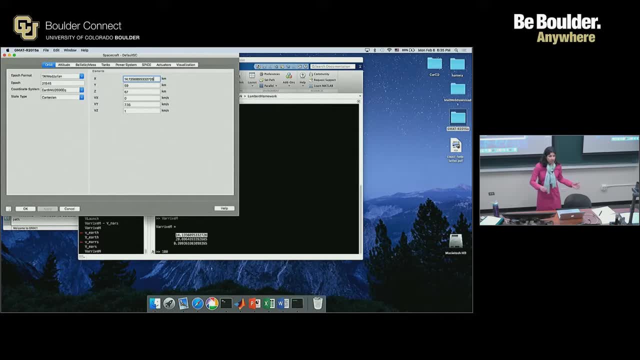 component to this really long number. So I'm just going to try and copy and paste it here. See how apply is still grayed out. I can click OK, but if I go back and look at that it's still 5,000.. So I was able to replicate it. If you want to do this copy-paste thing, you. 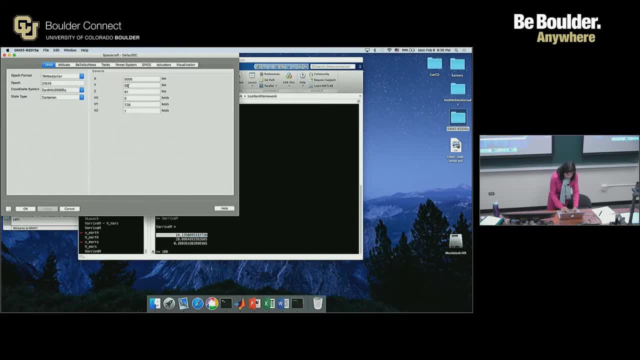 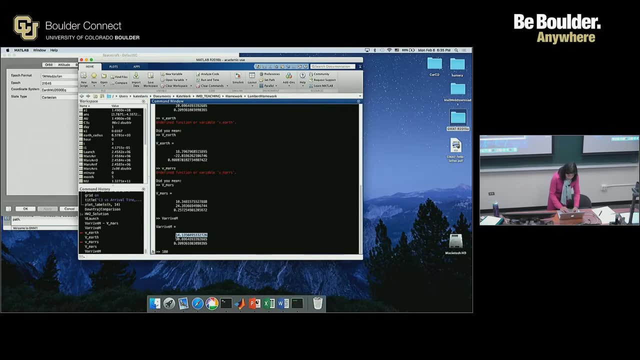 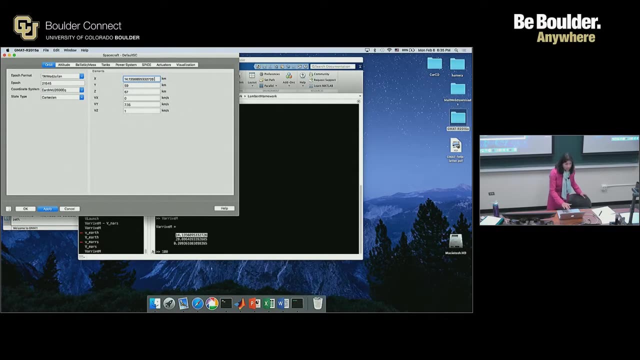 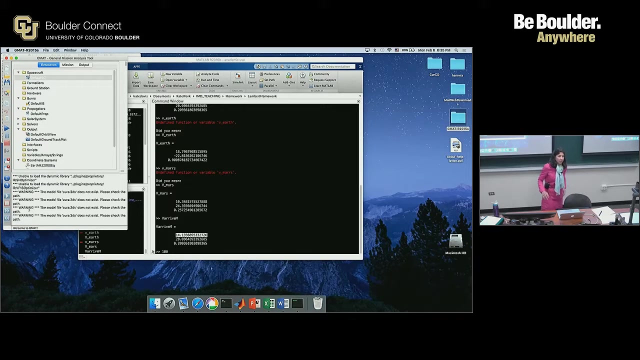 can. What I would suggest doing is when you copy it- oh there it was. So copy it and then add a keystroke at the end like a space, Just for whatever reason. put in a space, Then you can hit: apply okay, What some people were having trouble with? that? They thought 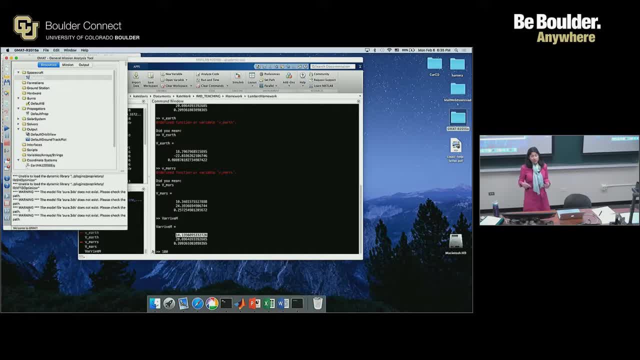 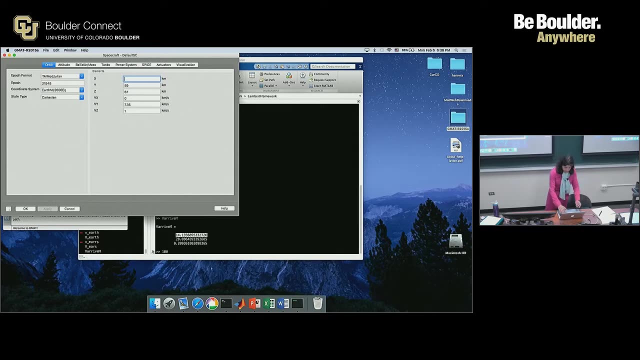 that they were actually putting in the right values, Okay, Okay, When in reality GMAT was not picking it up. A couple other things, just briefly. to talk about integrators, Let's just say that we were to put in a state of the spacecraft that 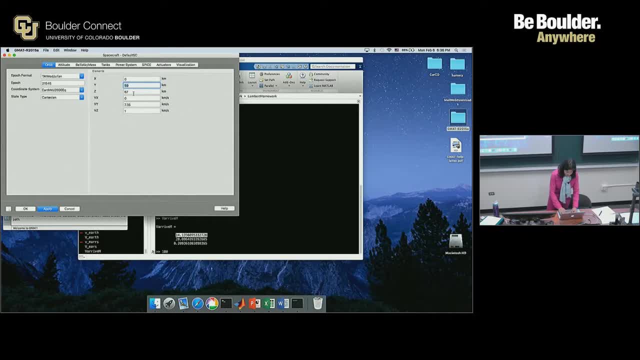 is now. this is in the Earth frame. okay, Let's just look at this. Let's just say we have these positions and these velocities with respect to the Earth. What does that tell you? Where are we In the center, Inside the Earth? Okay, Who has any idea what might happen if you try and throw this? 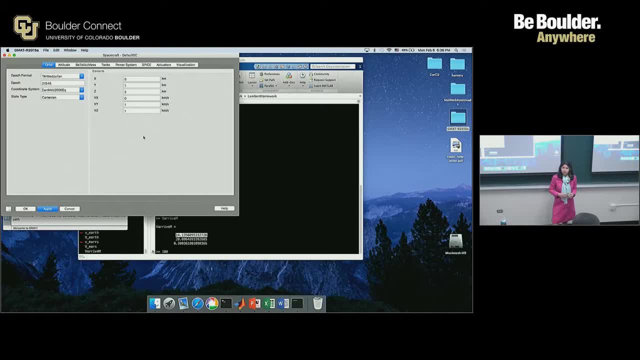 into an integrator, It won't converge. It won't converge. Yeah, When you're integrating, think about your force function. The force function that we have is something over a radius magnitude. Now, if your radius magnitude is very, very, 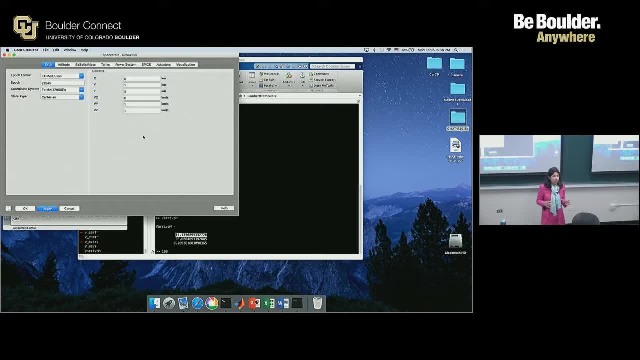 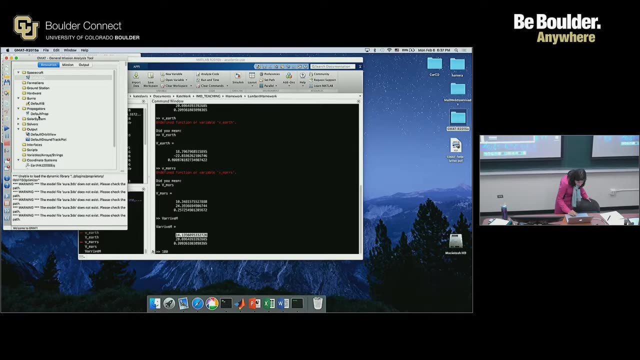 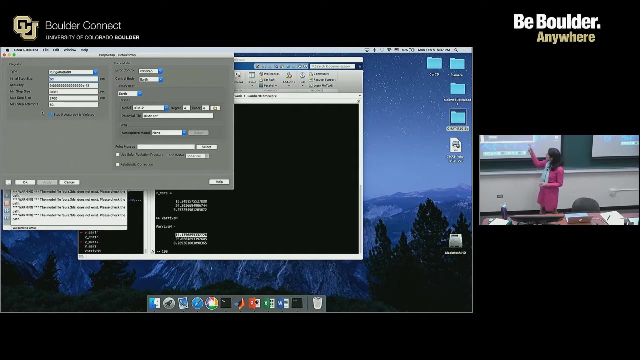 small. the terms in your integrator function are just going to blow up And what's going to happen is if you've got a really tight tolerance on your integrator. so if I were to pull up this default propagator, it's going to try and match steps to 10 to the minus. 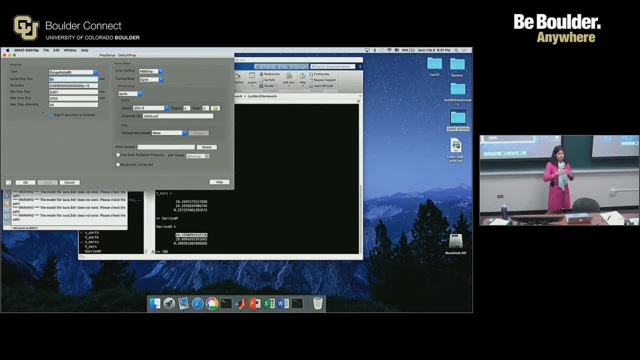 12. So essentially, what it's trying to do is it's looking at different steps of integration and it's going to try and get your successive steps to match to 10, to the minus 12. If you're inside the center of the Earth and you're kind of near a singularity, essentially, 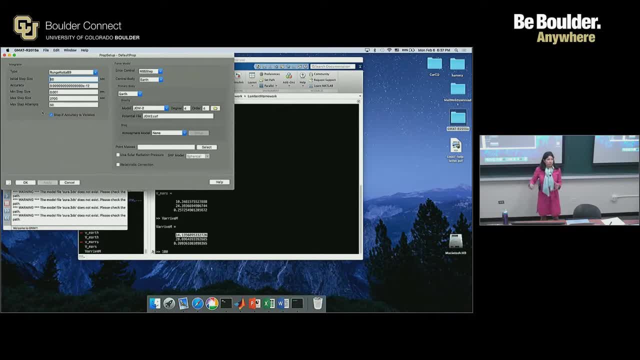 it's never going to be able to hit that, And so your integrator might start getting into an infinite loop. So if you're seeing really long integration times within GMAT, within STK, within MATLAB, with whatever you're coding in, and something is just taking really long, a long time to, run, you're going to have to figure out one where your initial position is, or you could also take a look and see: well, hey, I started way far away, but maybe I ran into something Like: maybe I accidentally am trying to integrate through Mars, Maybe my flyby is not taking. 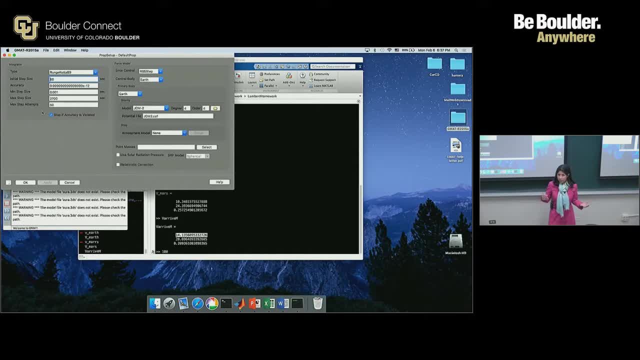 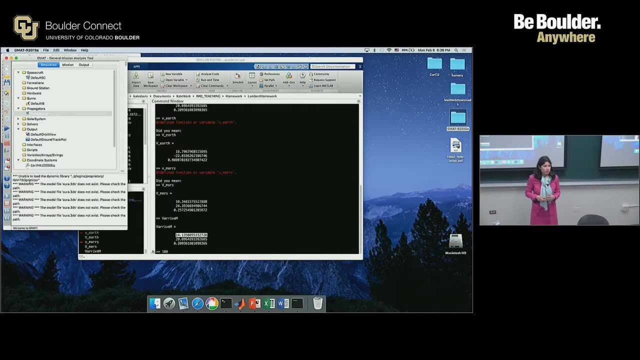 me over Mars like I thought it was. Maybe I'm actually going through Mars. So just a couple of helpful tips. Hopefully we'll save you guys some headache. Are there any other questions about the homework Or the labs? Yeah, I have a weird thing where my V infinity is actually negative for problem one. 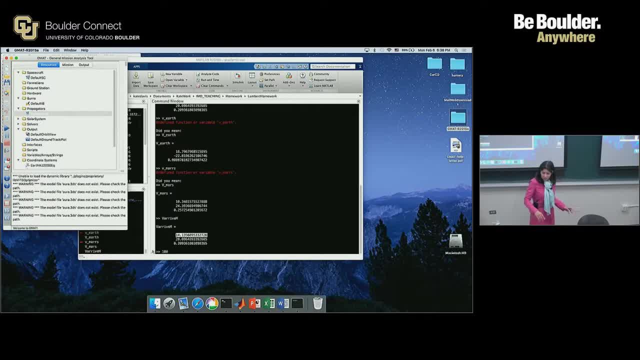 And so I don't know, I don't really know how that could happen. Oh, I sent an email just like a few minutes ago. Okay, Let me switch back to When you're taking your, When you're computing for V infinity, are you subtracting the components? 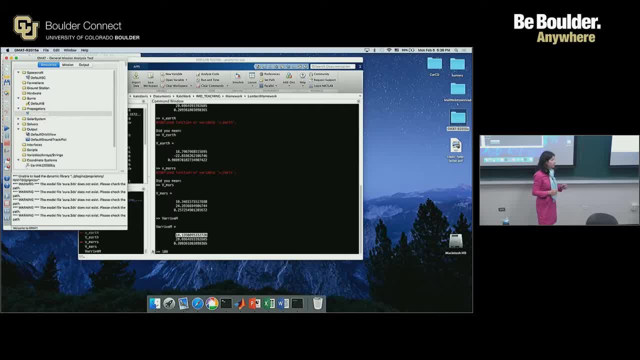 Or are you subtracting two different magnitudes? Two different magnitudes? I believe Yeah. So what you want to do is you want to subtractto, actually get V infinity. you don't want to subtract magnitudes, because then you're essentially just taking the difference in speed and you're 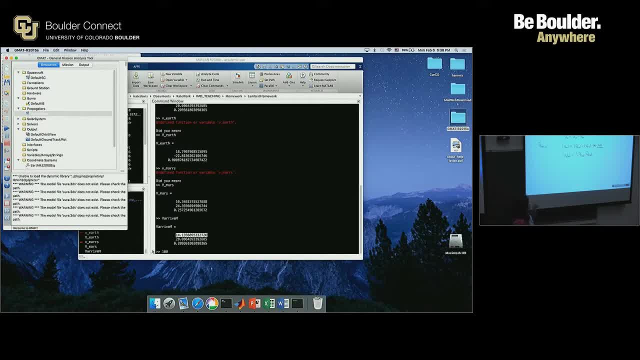 not taking into account the direction of the velocity. So to get V infinity, it's the magnitude of the planetary velocity minus thesorry, the departure velocity minus the planetary velocity, not the difference in two magnitudes. Okay, Welcome, All right. 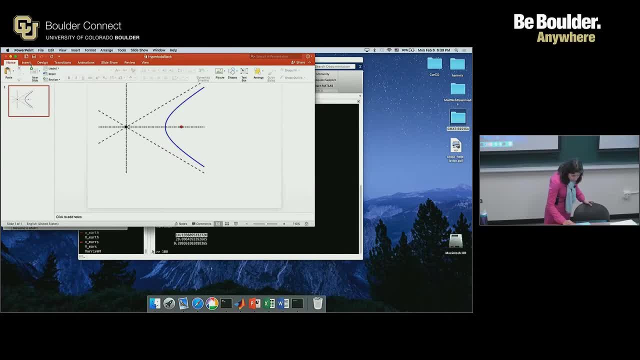 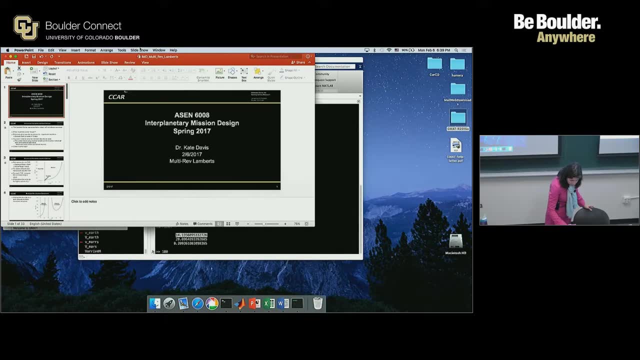 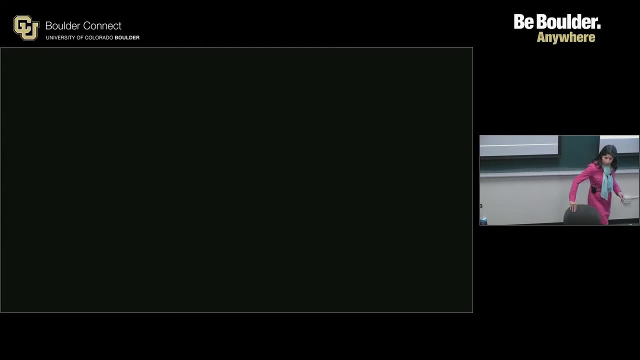 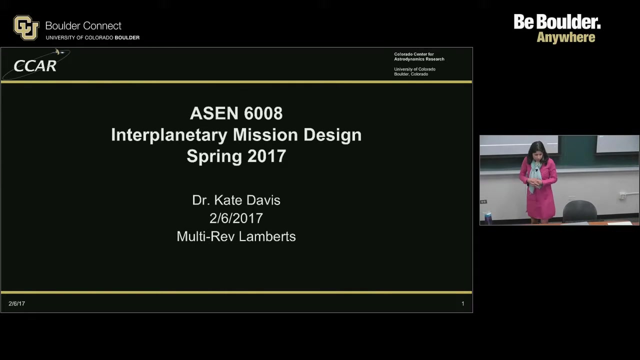 Not that one. We'll do that in a minute, Okay, All right, Pulled this up on both, All right, So hopefully you guys are, you know, enjoying this, So See you in a minute, Okay, Bye-bye. 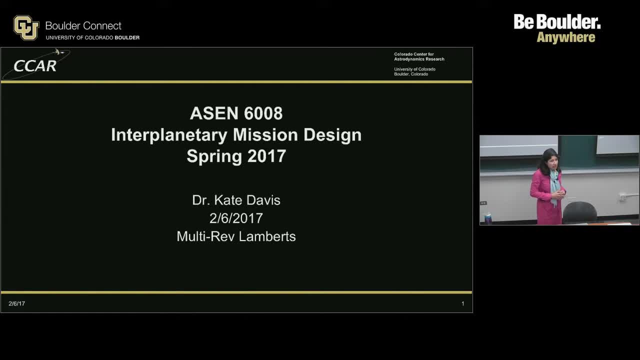 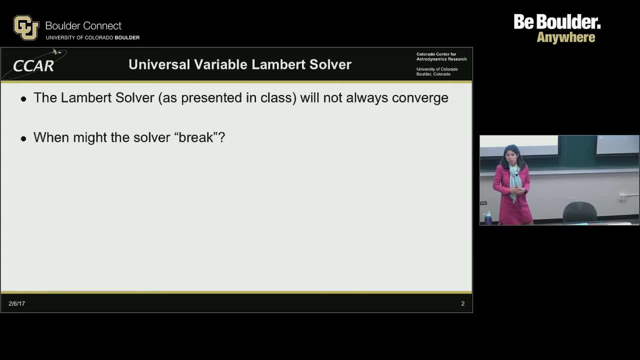 either have a working Lambert solver or you're really close to having a working Lambert solver. Now that I tell you that you have one, I am going to tell you that sometimes it will break. okay, Anybody have any ideas as to when the solver? 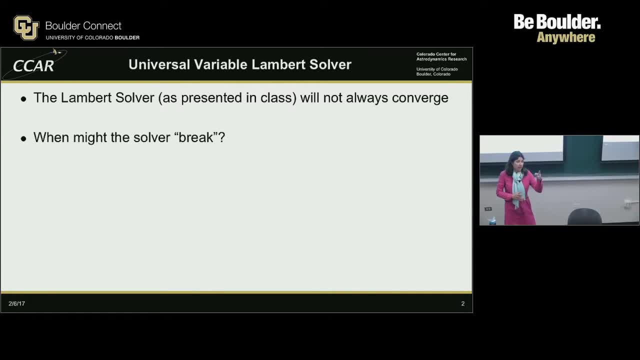 might break and why it might not. why it might not work. Yeah, If you give it a really small time of flight window and like one rev or more, then it'll break, because it's trying to go around the Sun in 30 days and then make it to Earth. Exactly exactly. If you try and say I want to go from Earth to Jupiter in one day or ten days, even it's not going to converge because, if you'll notice, it's looking at a difference in tolerance that's down to ten, to the minus fifth. 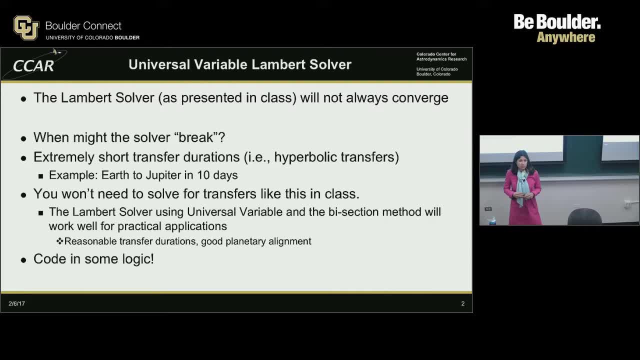 seconds and you're just not going to be able to find something like that. The good news is that I'm not going to ask you to solve for things like that in this class. Maybe it's an interesting academic exercise to see what a conic looks like. 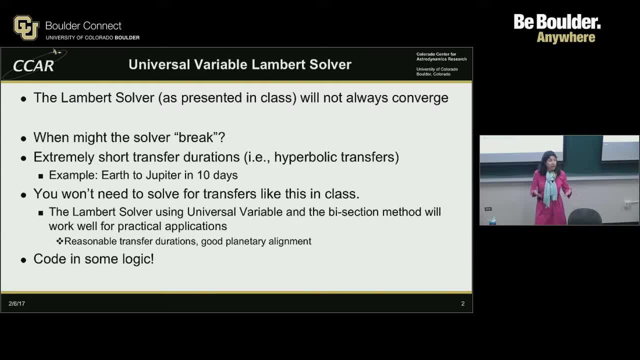 that goes from Earth to Jupiter in ten days. What kind of conic is that going to be? Yes, it's going to look kind of like a straight line. Yeah, it's going to be a hyperbolic. I mean you're going to need a lot of velocity to get out of the Earth, because I'm not going to ask you to do stuff like that. I mean, obviously you would need a huge C3 and there's not. there aren't going to be any missions that are going to do that. 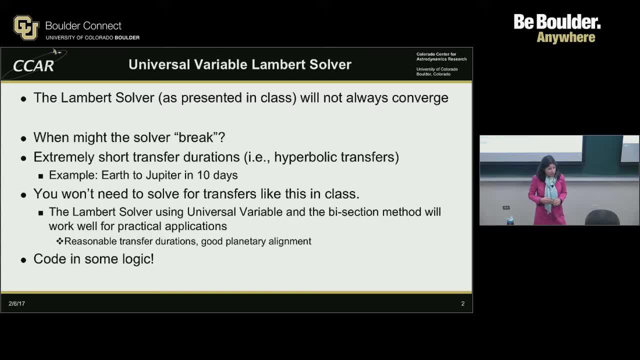 So this Lambert solver with the universal variable bisection method that we are using in class will work really well for practical applications And honestly we're mostly concerned with practical applications. NASA really doesn't want impractical things. They tend to be very expensive. I guess the 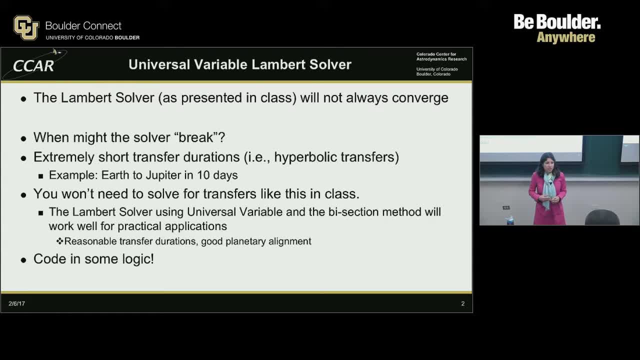 point of this is to code in some logic, You know. make sure that you're not looking at negative time of flights, for example, because it's really easy: if you're going through a for loop, it's going to be a for loop. 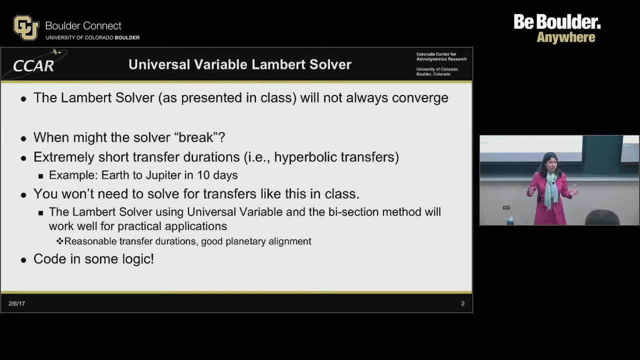 and you're trying to look at, you know, different planetary alignments. it might be really easy to accidentally like if you're cycling through a whole bunch of launch dates and a whole bunch of arrival dates, especially for an Earth to Venus transfer, it might be really easy to accidentally. 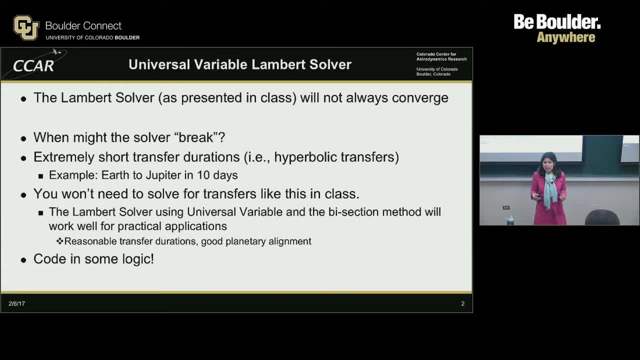 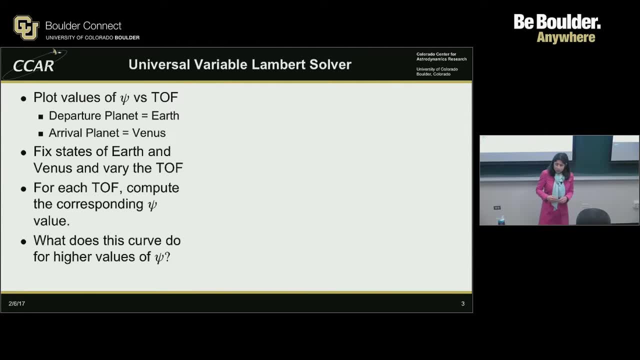 come up with a negative time of flight. Just pay attention for those sorts of things and make sure that you don't have that in your code. Okay, so one thing that is really interesting to do is plot values of the variable psi versus time of flight. 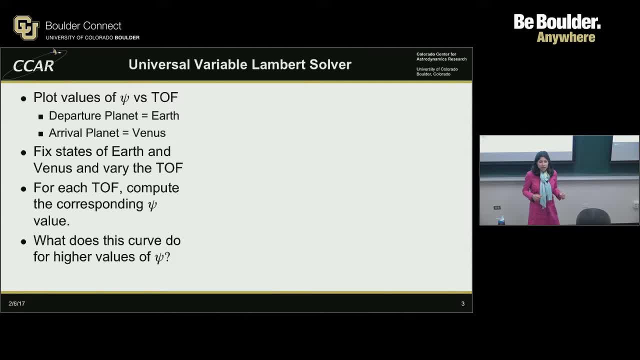 So one way to do that is, let's just say, we pick a departure planet of Earth and an arrival planet of Venus. Now what we're going to do is based on those states. now we're not going to let those states move. we have a position of Earth. 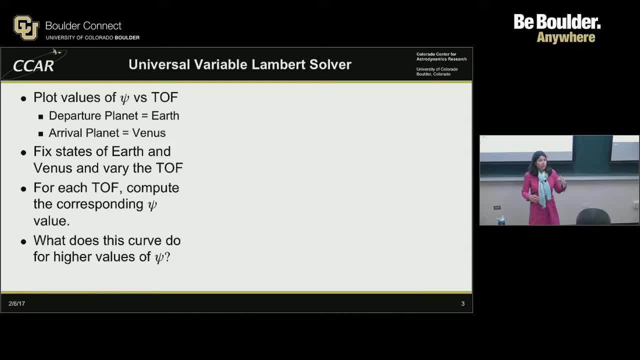 we have the position of Venus, where now we're going to vary the time of flight and look at what different conics might look like based on those two positions. okay, And for each time of flight we want to compute a corresponding value of psi. 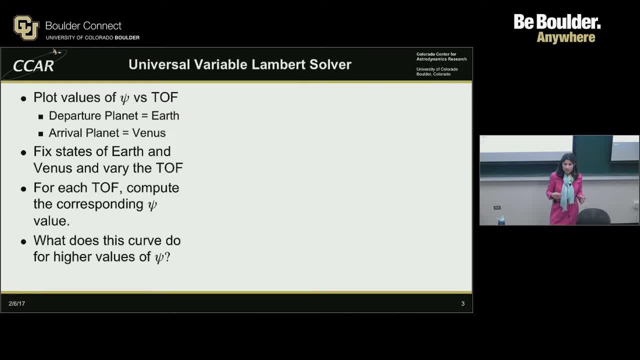 And remember, psi physically represents delta e squared. So this is what that plot would look like. Okay, So we've got psi squared on the bottom and on the y-axis we have time of flight in days And for delta e or delta e squared, or psi values, 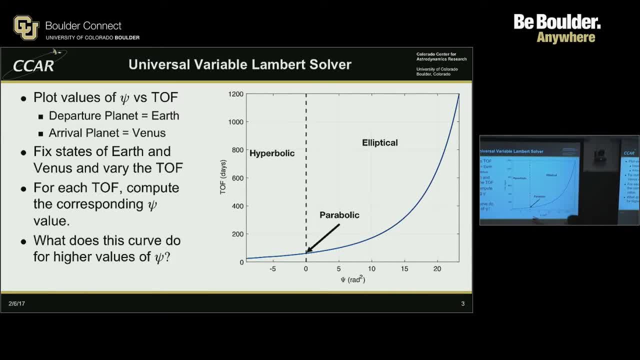 that are negative, we're looking at hyperbolic transfers. If psi is exactly zero, it's a parabolic transfer, And if psi is positive to a certain extent, we've got an elliptical transfer. So what do you think this curve does at higher values of psi? 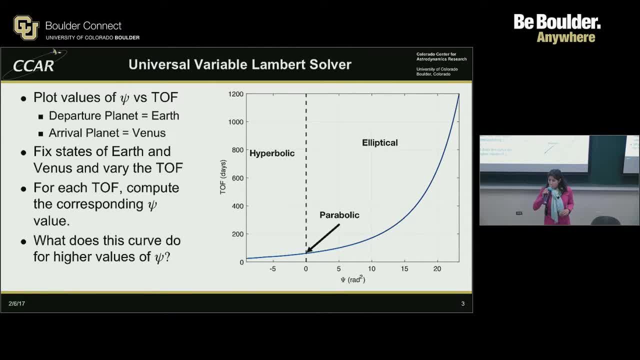 It circularizes everything. Like, can it become a circle? Like, if you have a value for parabolic, is there one for a circle? Like, is that a thing? If you have, like, high enough phi, is that what it is? 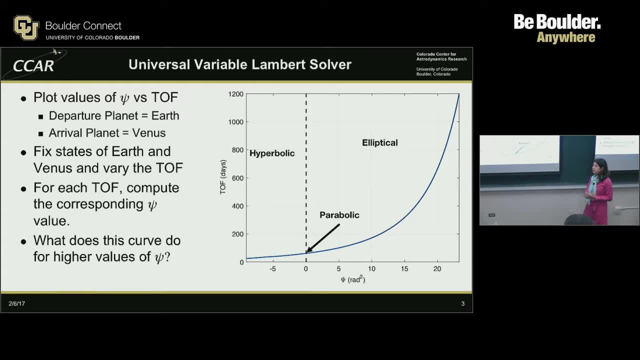 This is like strictly out of curiosity my part. I would have to think about that. I don't know if you can ever approach a perfectly circular transfer because you're not starting and ending at the same radius. Okay, Because you know you've got different initial and final. 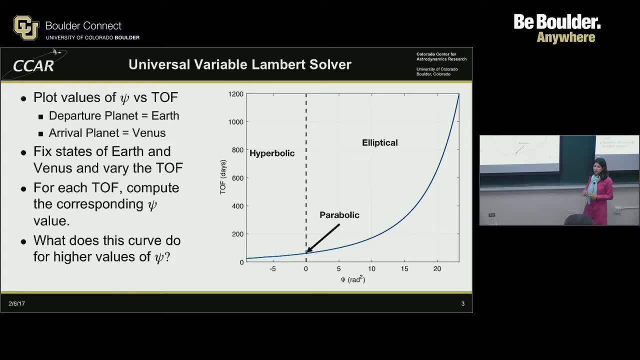 radii about the sun, And so I don't think you could ever have a circular transfer. Okay, Anybody else? Yeah, I was just thinking strictly. psi is only delta E squared in the elliptical case, right, Because you can't have a square root of a negative. 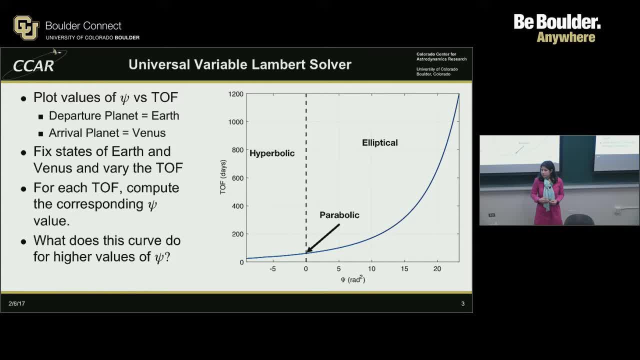 So I think Vellato defines some other M or something for the Yeah, yeah, For this universal, for the way it's formulated. if you get a negative value, then you're looking at a hyperbolic orbit, But if you think about, you know, delta E. 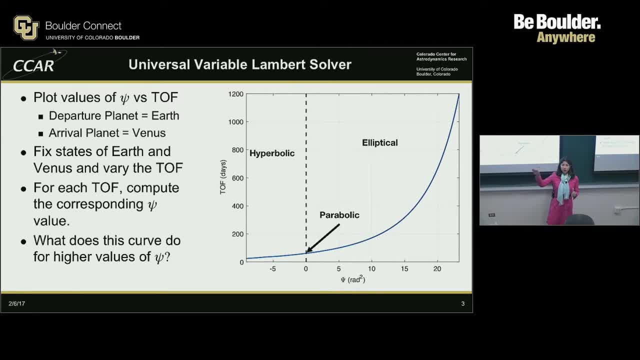 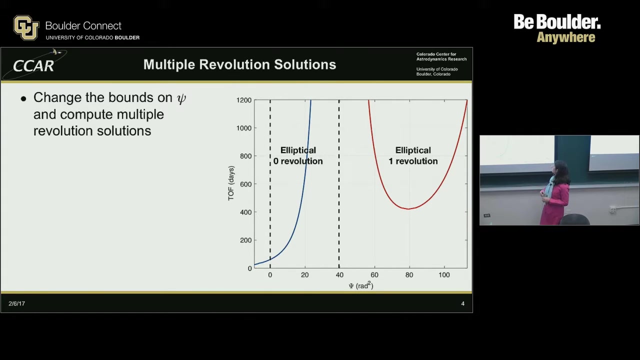 you're looking at how delta E changes around. So if, if psi is getting higher, that means delta E is getting higher. What are we looking at? Are we going to have multiple revolutions? Yeah, Multiple revolutions. So this is what we're looking at. 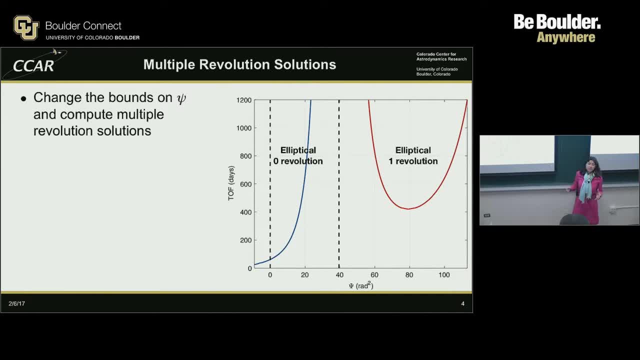 If we extend our plot, so let's think about it. If we have a transfer that is a bound on a single revolution, transfer, right? How many degrees is that? 360, right? So in radians, what are we looking at? 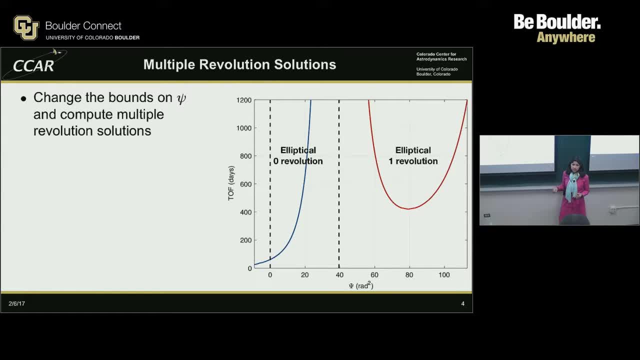 2 pi. 2 pi squared is Well, 4 pi squared, right? That's essentially this bound right here. So as we get above 4 pi squared, we're looking at these elliptical one-revolution solutions, So we can. 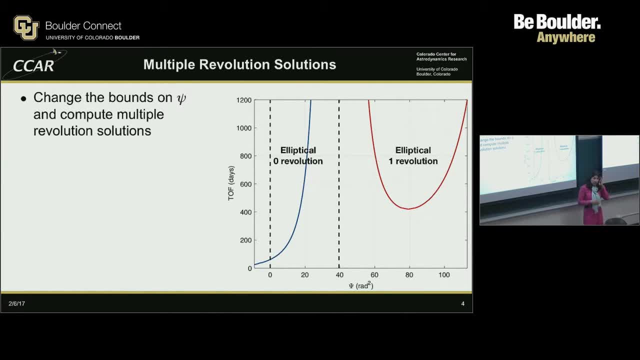 in the initial Lambert solver that we had. does anybody remember what, at the beginning, we initialized values of psi? Does anyone remember what our initial values for psi, low psi, up and our initial value of psi were? Minus, minus pi squared and plus pi? 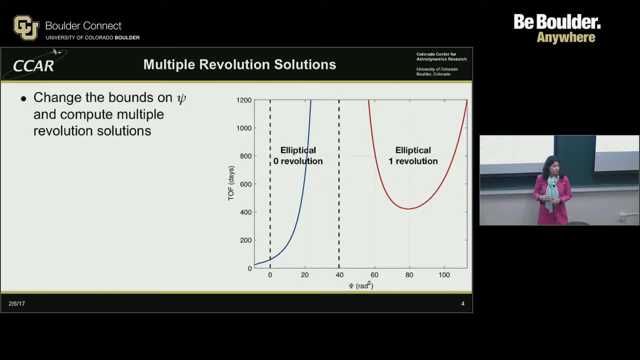 Plus 4 pi. sorry, Yeah, Minus, 4 pi squared and plus 4 pi. Yeah, they were essentially these bounds Minus, I think it was minus pi, or minus pi squared and 4 pi squared. That way when we're doing a bisection method. 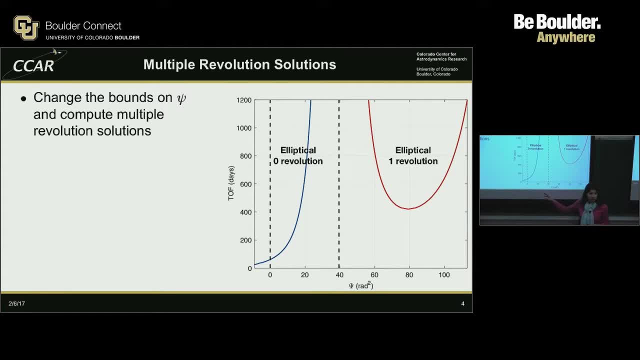 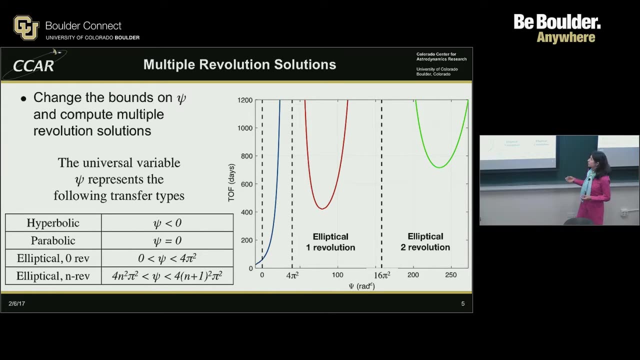 we're guaranteed to get something in here. Now, if we want to extend our search to multiple revolutions, then we need to change our initial values on psi within the Lambert solver And we can actually get you know 2,, 3, 4 revolution solutions. 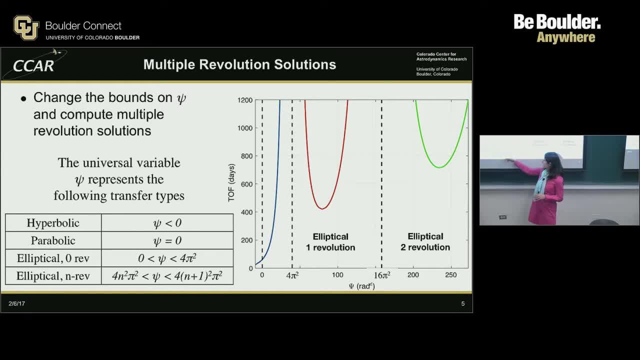 And so the universal variable psi basically represents the following types. If we aren't going to full revolution, psi is going to go from 0 to 4 pi squared, and then it scales with n for each rev. And so you could. so here's 16 pi squared. 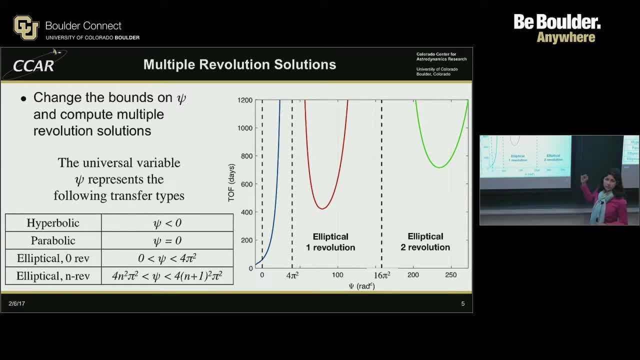 and then you could just go on and on for different, for, you know, extending 3 rev solutions When a 3 rev solution would ever be useful in interplanetary mission design, I don't know. I mean, that's going to take a lot of time. 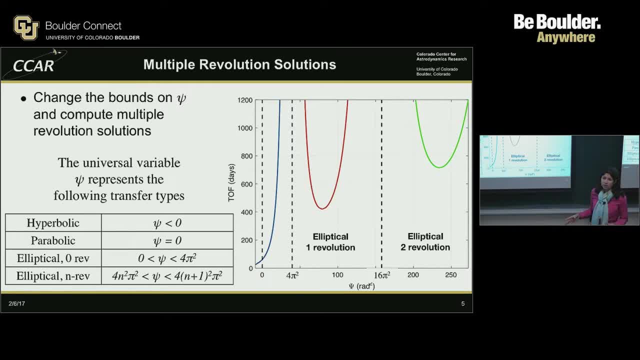 It's interesting to think about, maybe interesting to compute and see graphically what it looks like, but it's probably not something that we would want to do because it's just going to take so much time. So now we see we've got more. 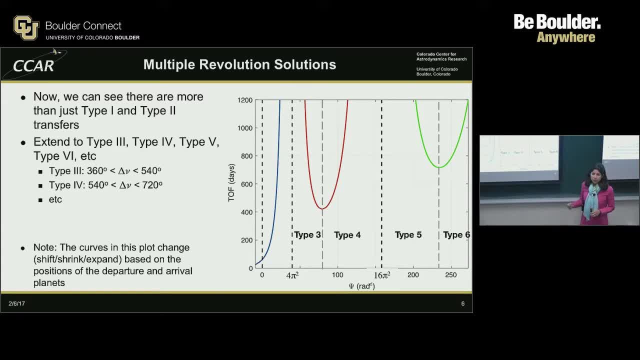 than just type 1 and type 2 transfers. Now we've got type 3 and type 4, where type 3 is going to go from basically 360 to 540, and then type 4 is going to go from 540. 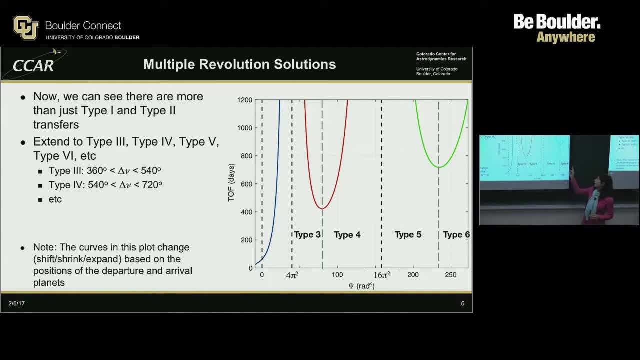 up to 720, and then type 5 and type 6,, basically just incrementing in segments of 180 degrees. Does that make sense? Okay, And one thing I did want to note is the curves of this plot. the basic shape is going to stay the same. 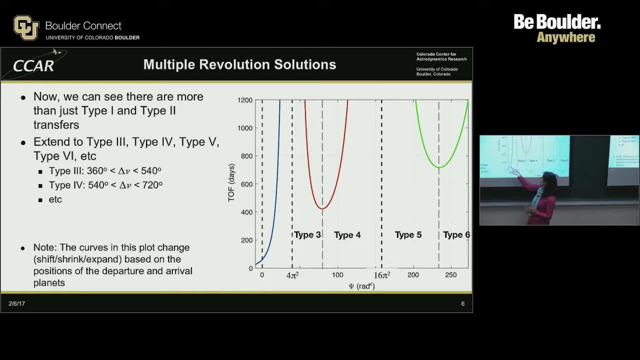 where you've got, you know, this kind of almost parabolic or hyperbolic looking shape here and then kind of you know almost parabola-like shapes. They will shrink or shift or expand based on the different departure and arrival points. Because you know obviously where you actually have a hyperbolic time of flight is going to be different based on the positions of the planets, So different books are going to use different nomenclature. Unfortunately, there's no set standard. 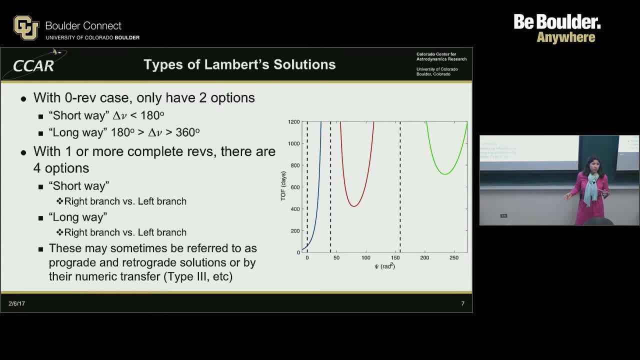 So sometimes, like with the zero rev case, we can refer to it as the short way or the long way. you know, essentially type 1, type 2.. But with one or more complete revolutions there's basically four options. You can go the prograde way around. 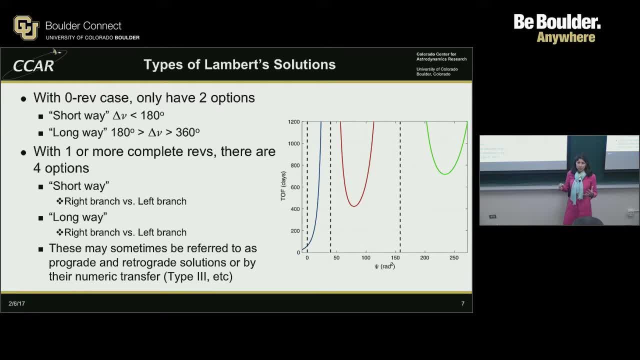 where it's the odd type transfer, like type 3, type 5, or you could go the retrograde way around the orbit where there's type 3, type 5.. Or you could go prograde, So you've got prograde, retrograde. 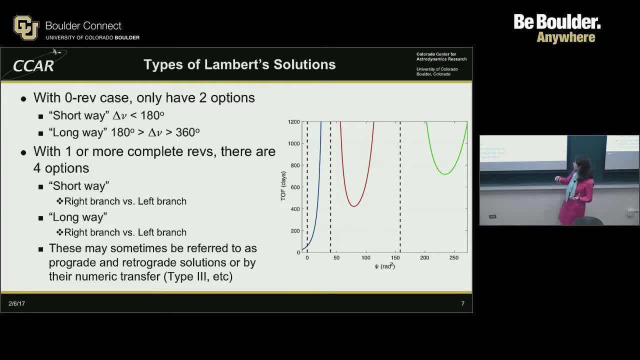 even or odd type transfer So you could have transfers over here that go prograde or retrograde, Transfers over here that are prograde or retrograde. Hopefully that kind of makes sense In this class. I guess some people refer to this. 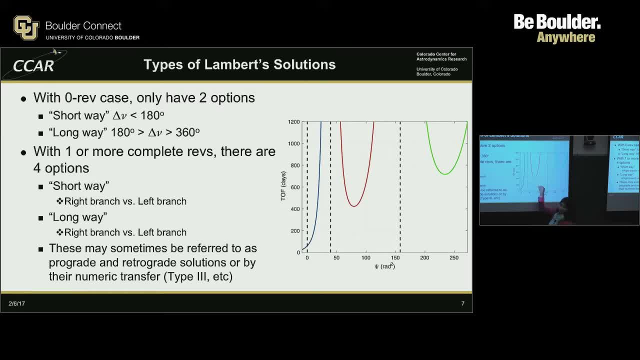 as, like your left branch solution and your right branch solution, Different. I forget what Bate, Mueller and White refers to them as In this class, we're simply going to do type 1, type 2, type 3,, type 4.. 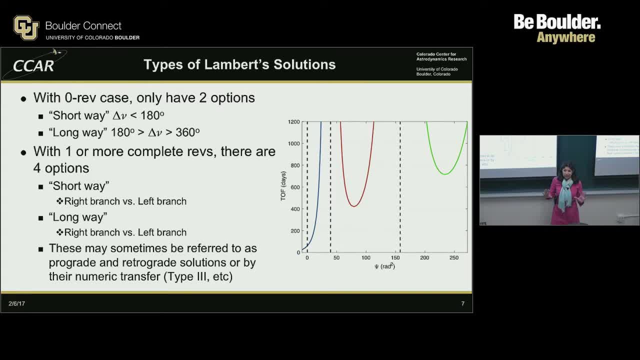 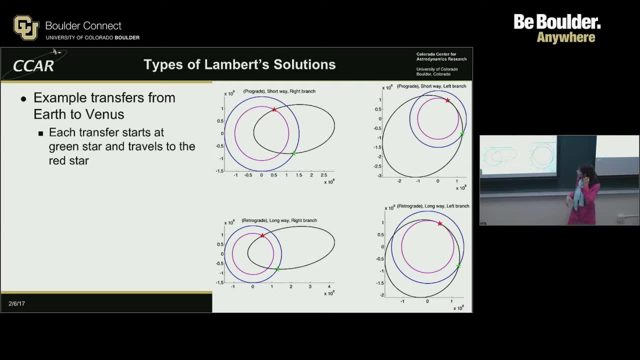 And we're always going to assume prograde motion. We don't really need to mess with retrograde solutions. They are kind of interesting to look at though, So here are some example. transfers from Earth to Venus. Each transfer is essentially starting at the green star and going to the red star. 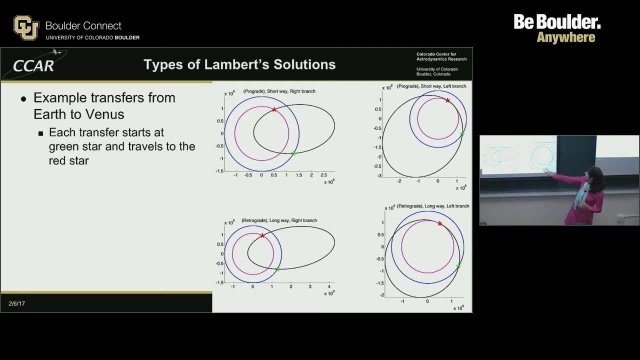 And so I've got the prograde solutions on top and retrograde solutions on the bottom. So because I can't reach the top, I'll just kind of demonstrate this. So if we were going retrograde from Earth to Venus the long way around, 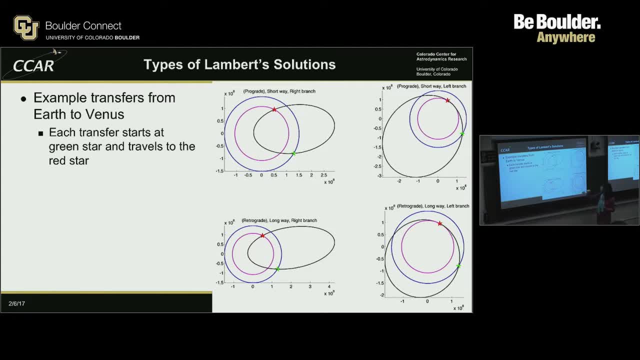 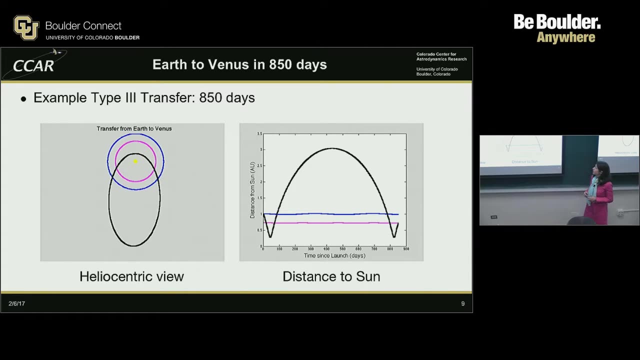 we're basically going like this And if we're doing retrograde, the long branch here all the way around and back. If you want to look at a type 3 transfer, this is kind of what it looks like. Here's the type 3 transfer. 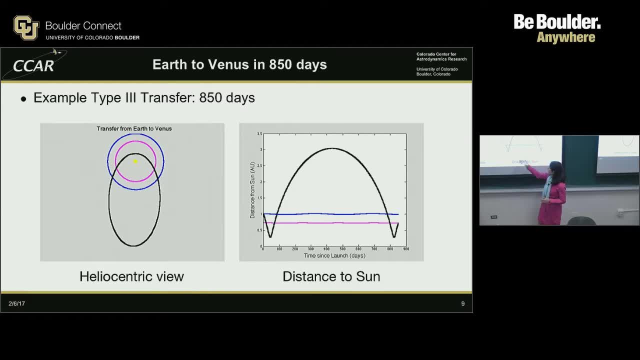 from Earth to Venus. It takes 850 days. So I've also plotted the distance to the Sun so you can kind of see what's going on. So basically we start at the Earth, we cross Venus' orbit and then most of the transfer. 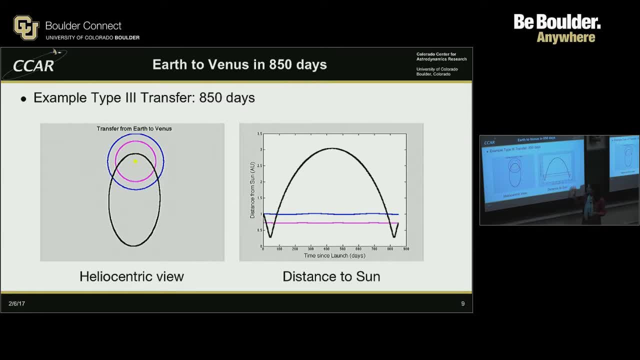 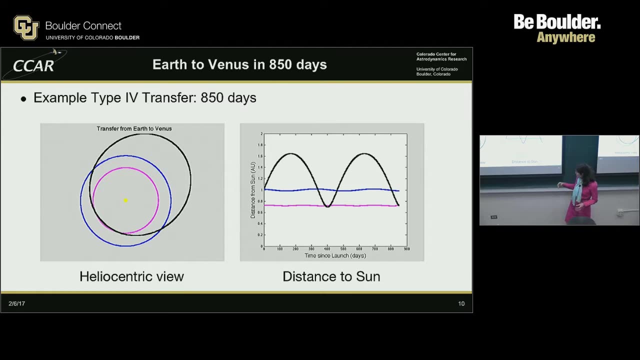 basically from 100 to 800 days. 700 days are essentially on this really long portion where you're going really slow And then you eventually get back to Venus. Here's the type 4 transfer that takes 850 days. Again, we've got our heliocentric distance. 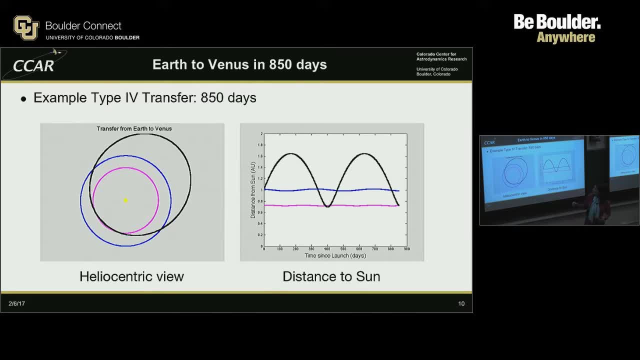 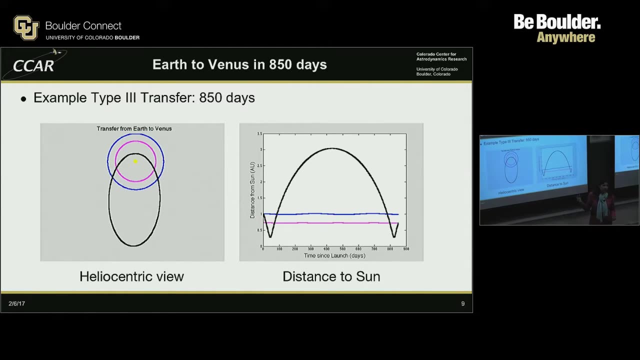 and the distance to the Sun. This one, you can see it looks much more feasible than the previous one. Now, this previous solution, you're really burning against the direction of the Earth when you're departing and you're not really hitting Venus at a tangential direction, right? 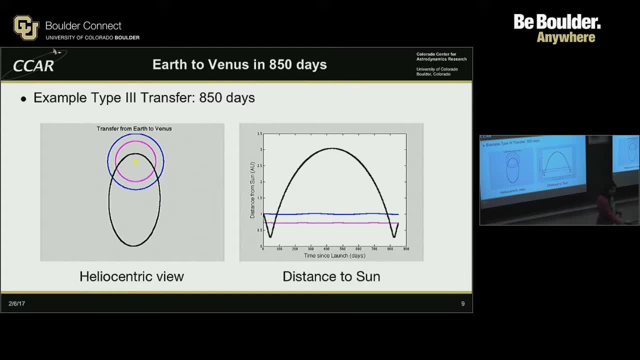 It looks like a pretty crummy transfer. if you wanted to use this for interplanetary mission design, This one not so bad, right? I mean, look how tangentially you're kind of coming into Venus And here you're leaving pretty decent. 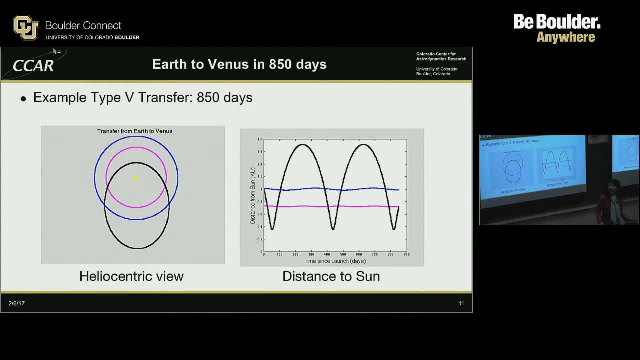 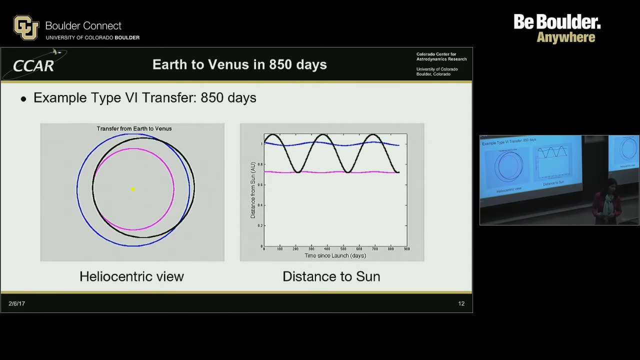 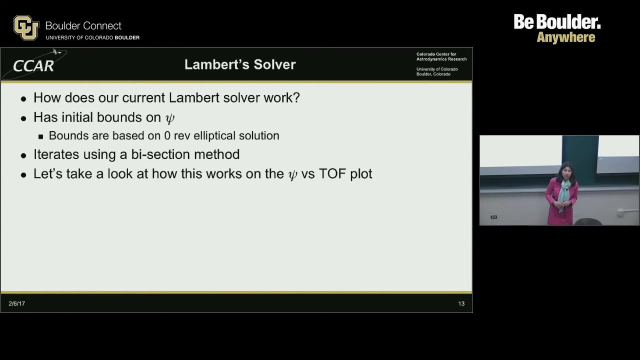 with respect to Earth. Here's a type 5 transfer. So this is where you're making two revs- Again not that useful, Kind of interesting to look at- And a type 4 transfer for 850 days. So the way that our current Lambert solver works. 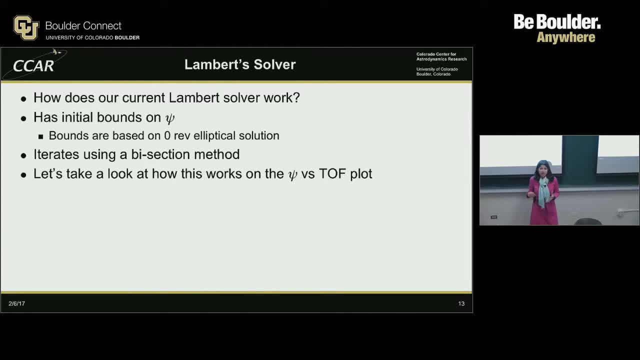 is, it has initial bounds on psi And it's completely based on the zero rev solution. That's what we kind of described, And we're iterating using a bisection method. So I kind of wanted to take a look at how this works. 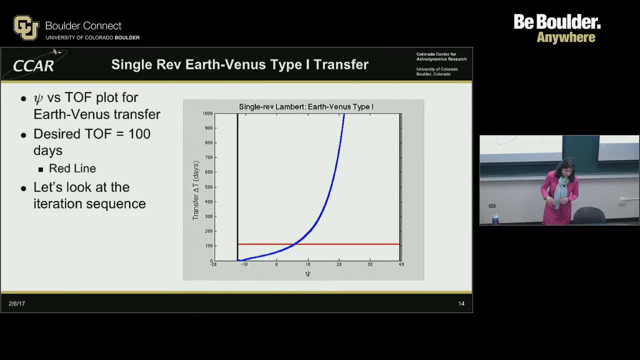 on a psi versus time of flight plot. Okay, so here's the single rev: Earth to Venus transfer. Let's say that we want to converge. We know that we want to get from Earth to Venus in 100 days, So I've kind of represented that. 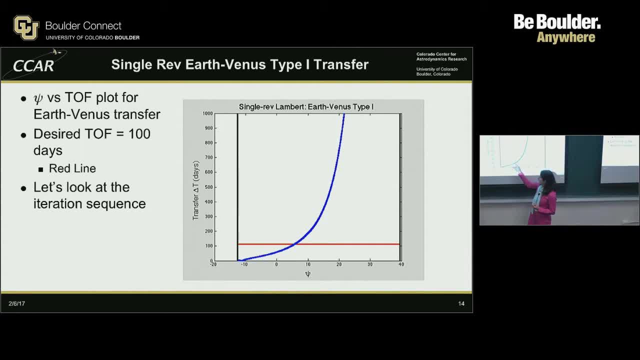 by this red line. So we're looking for this psi value. Okay, so if we were to look at the iteration sequence, it might look something like this. So our initial guess. if you remember, we initialized it as zero. So here's the first guess: zero. 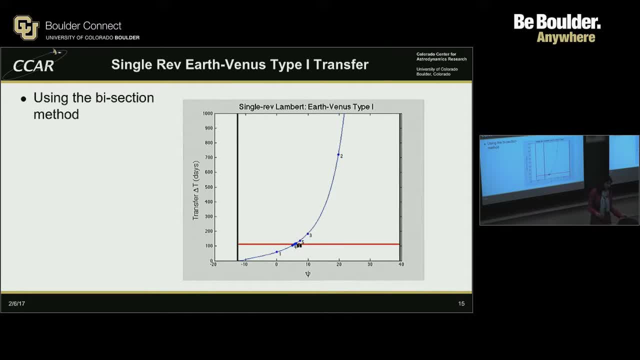 Obviously that's too low. So what it's going to do is it's going to take half of this distance here, Remember, it's psi up plus psi low, divided by two. So now we get part two and this section is essentially rejected. 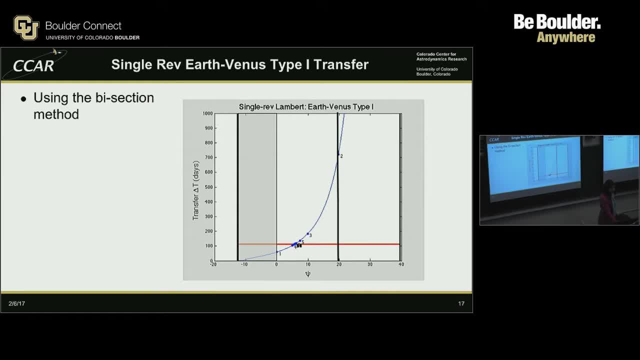 for where the solution might be. And then point two is obviously way too high. That time of flight is, you know, roughly 800, where we're looking for 100 days. So it'll get rid of this region and pick something in the middle. 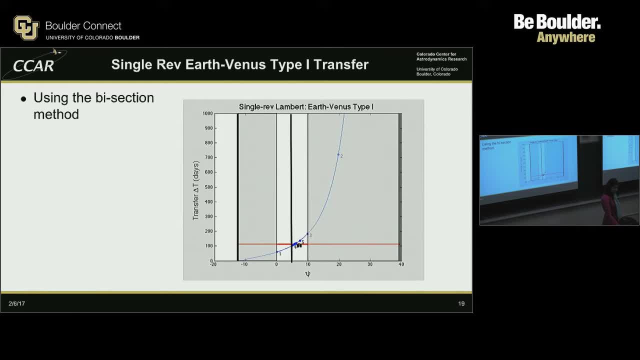 at number three, And we kind of keep going from three, four and we essentially, you know, essentially, we're just getting closer and closer to the solution, you know, cutting our step size down. Now to read to time: 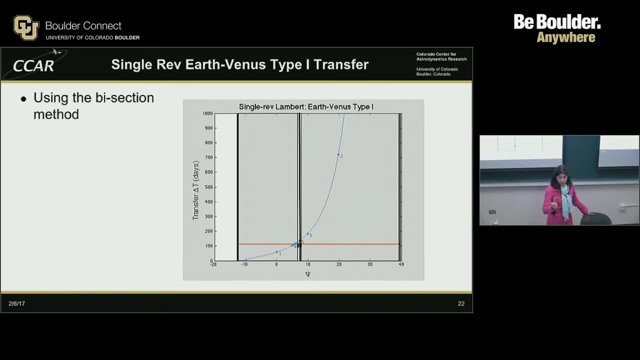 we set the tolerance at 10 to the minus fifth seconds. We want our time, the time we're computing within our Lambert algorithm, to match our desired time within 10 to the minus fifth seconds. If you think about that, it's pretty tight tolerance. 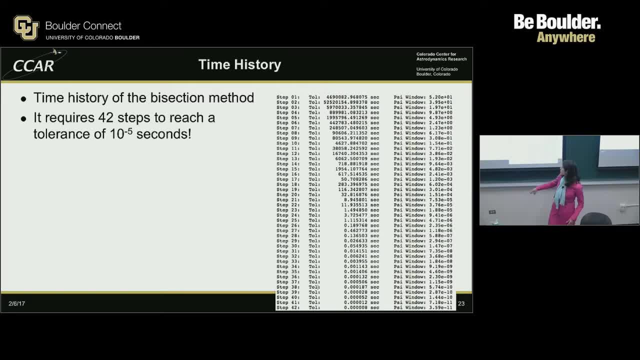 And it took 42 steps to get there. And this is just a history. So at the very beginning, you know, we were obviously off by seven, 800 days, you saw. But after you know, 42 iterations, we're down to that. 10 to the minus fifth tolerance. Way back in the day, that was when computing time was actually, you know, more at a premium than it is now. This was an issue, So some people wanted to use a Newton-Raphson method for speed. 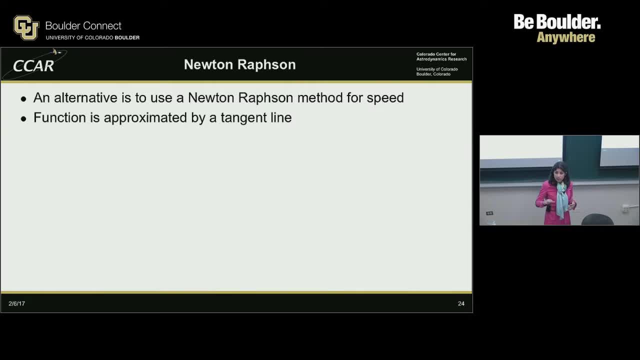 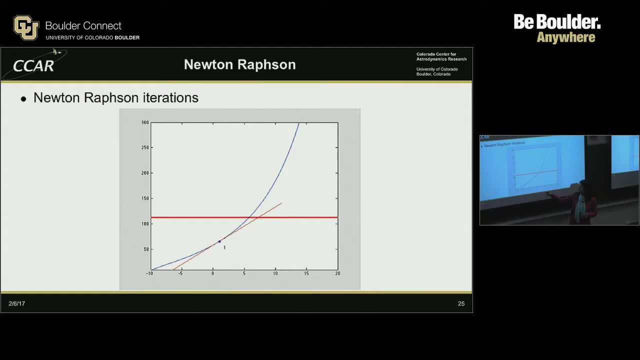 And the function there is approximated by a tangent line. So if we look at the same curve, you look at your initial starting guess and you approximate the slope there as a tangent, and then you can look at different tangents until you narrow in. 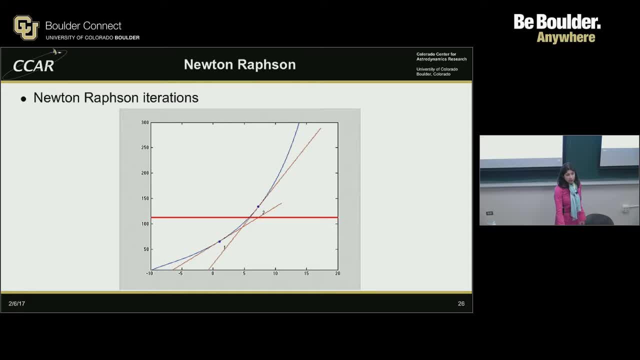 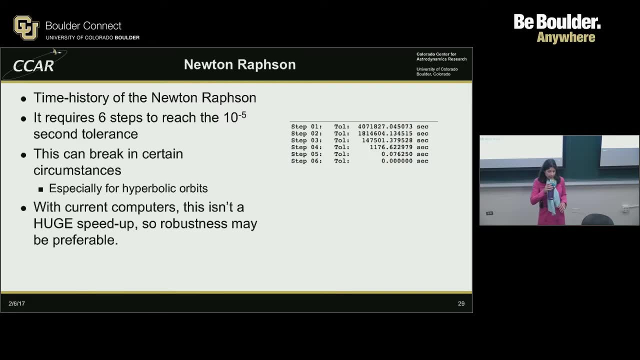 So we see that that tangent's not where we want. So now we're up above This. one only took six steps to reach the tolerance. The problem is that this can break in certain circumstances even more easily than the bisection method, especially for high-frequency. 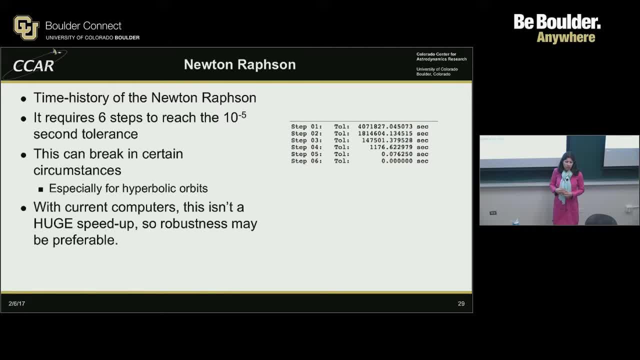 or hyperbolic orbits And with current computers it's not really a huge speedup. so the robustness factor, you know, might be preferable to this If you want to speed up your code in the future and you know that you're going to be. 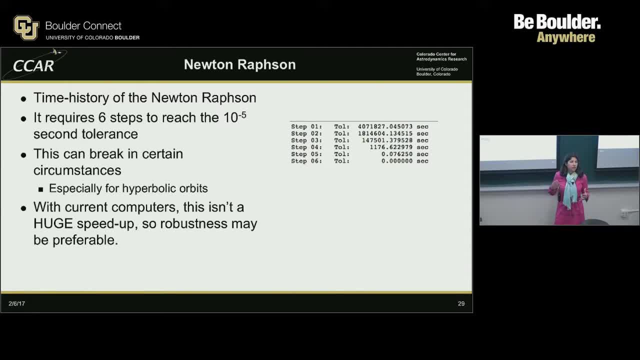 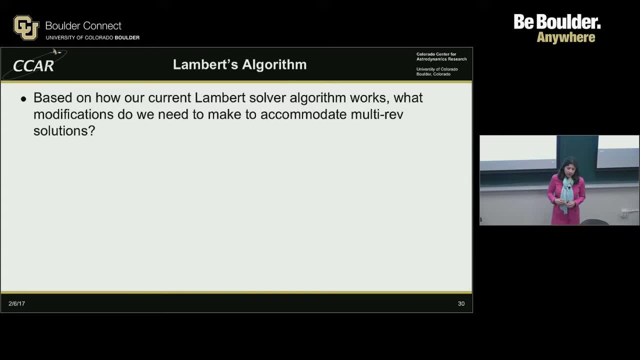 in elliptical regions and you're going to be computing a lot of data. this is something you might want to take a look at. So, based on our current Lambert solver, we need to make some modifications to account for multi-rev. So, first, what do we need to do? 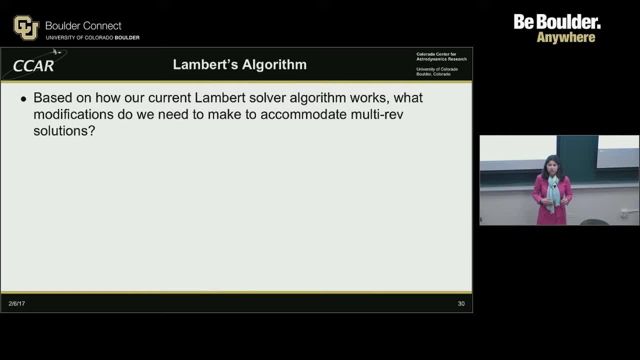 Increase the psi-up boundary. Okay, we need to increase the psi-up boundary. What else We have to tell it how many revs we want it to look for. Yeah, we probably need to tell it how many revs we want it to look for. 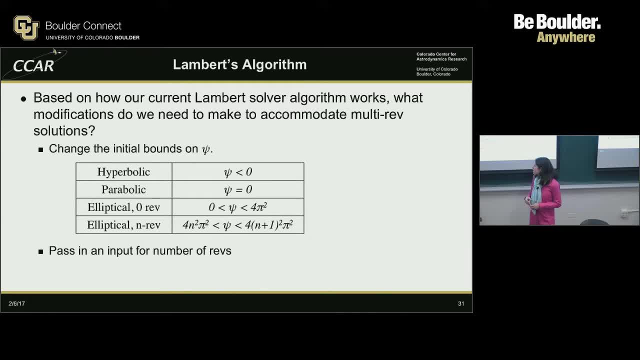 Okay, so we want to change our initial bounds on psi and then pass in an input for the number of revs. Does anyone remember what the curve looked like for multiple revs? Well, let's talk about the curve for the single-rev solution. 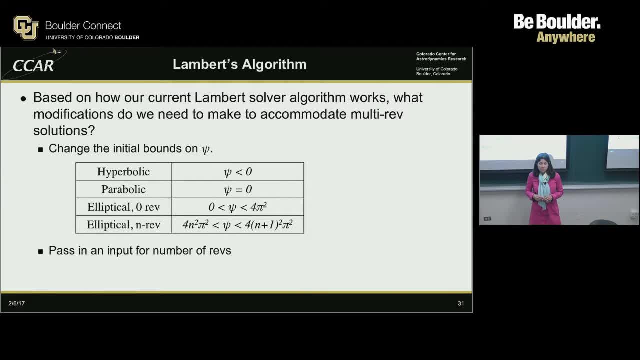 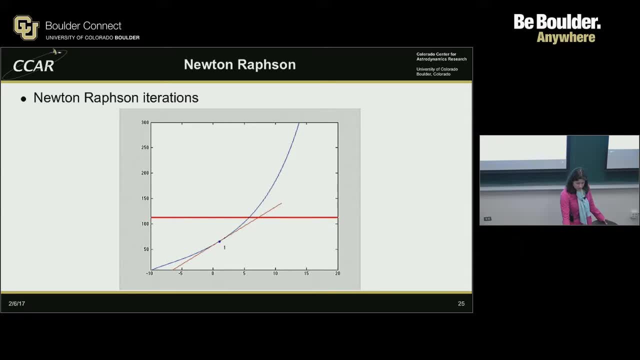 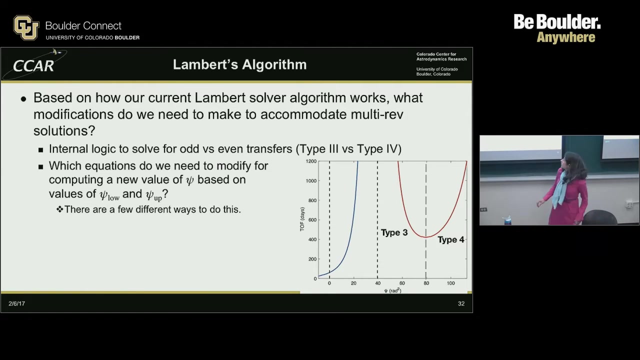 What's the slope For that single-rev solution? let's go back to. What's the slope of this curve? It's always positive. What about our multi-rev solution? It's negative at the beginning, So you're going to want to put in. 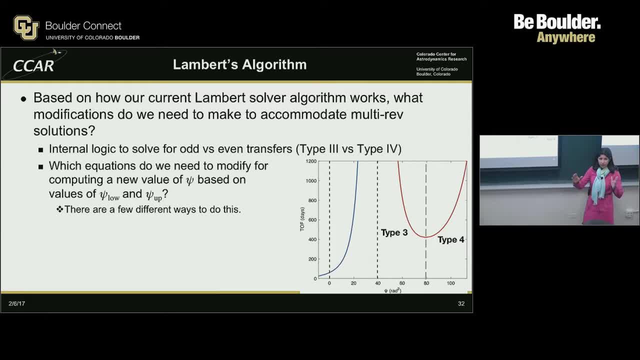 some internal logic, because obviously that bisection method, taking psi-up over psi-low, is not going to work for this type 3, or this type 3 transfer. It's going to work on the even side but not on the odd side. 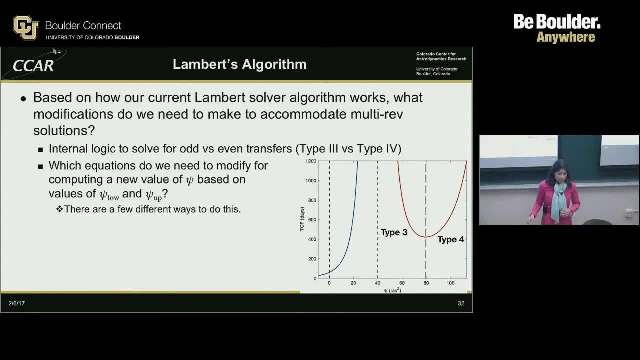 So you're going to want to put in some internal logic to. It's up to you how you do this. There's a few different ways to do it, But basically a good way might be to pass in the number of revs and whether you're looking for. 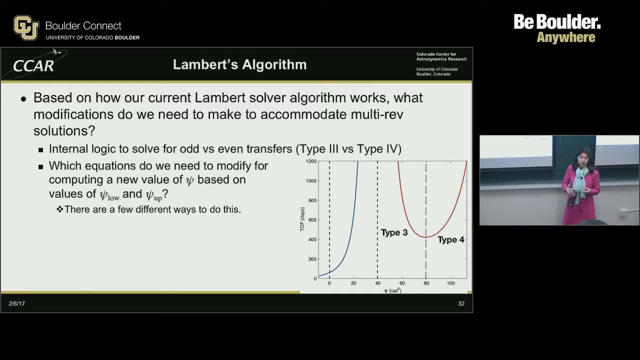 a type 3 or a type 4 transfer. Once you have that, then you can figure out which equations you want to modify on the psi-up, psi-low front Basically to make a negative slope rather than Basically you're looking for. 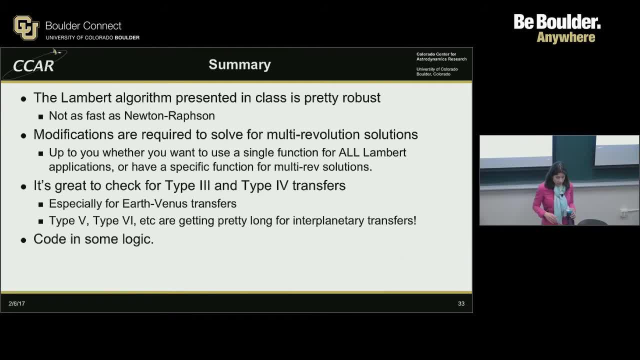 the negative slope instead of a positive slope. Okay, so just in summary, the Lambert algorithm presented in class is pretty robust. It's not as fast as a Newton-Raphson method but with, like I said, with computers, computing power these days. 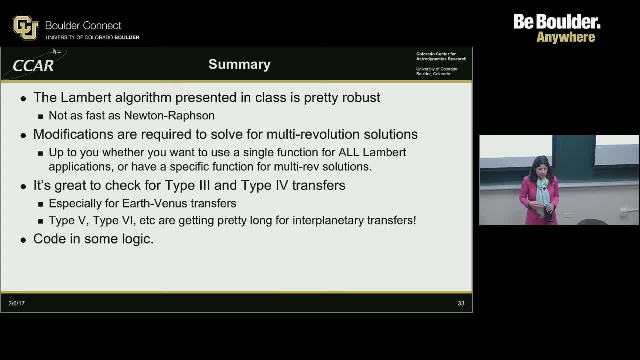 it's fine. There are some modifications that we need to do the multi-rev solutions. It's up to you completely whether you want to have one function that will do all cases or have a function for zero rev and a function for multi-rev. 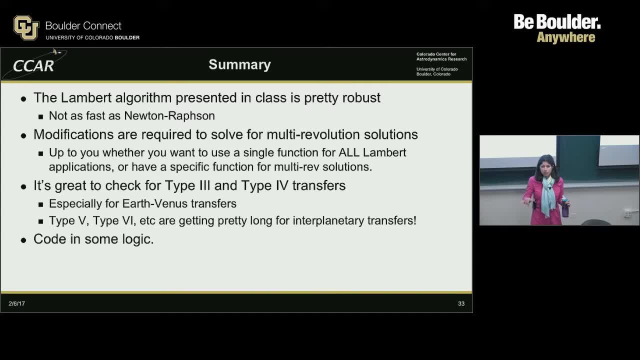 Completely up to you. I personally have two different functions because I don't like to have a lot of if statements within my code. I think it slows it down, especially if I'm searching over large portions of data And when we're looking at let's say, the final project and you're looking at transfers out to Neptune. you're not going to be looking at multiple rev You may need. There are some really great transfers that use multiple rev solutions from Earth to Venus, because you can wait for Venus. to get into good alignment and it doesn't take that long. You might spend an extra 80 to 100 days, but if you're going to cut your C3 by 10 or in half, then it's very useful. It's great to check for the type 3. 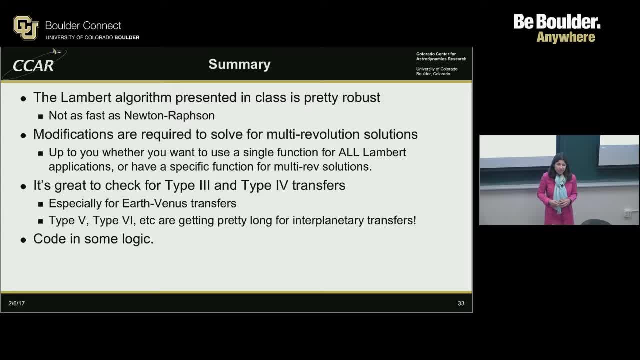 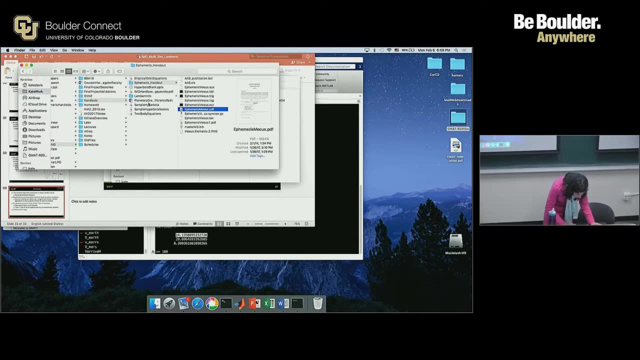 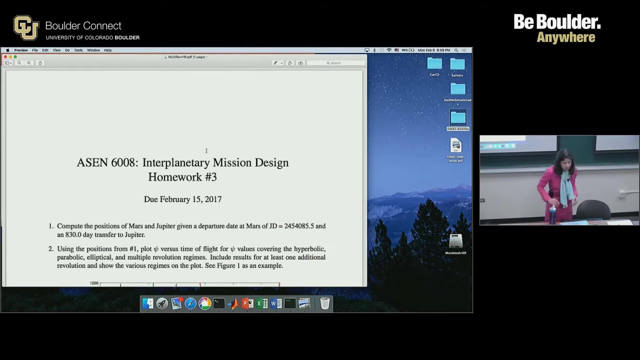 and 4 transfers, but it's getting long for most applications. The homework for this week. Let me see if I can pull that up. You're going to compute the positions of Mars and Jupiter based on certain dates and I want you to create 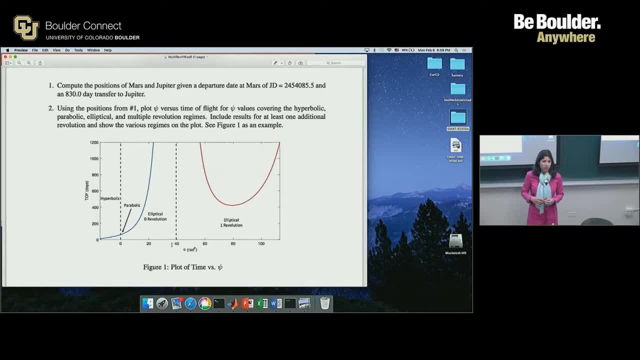 a plot like this, this multi-rev plot, The psi versus time of flight, and show the different regions on the plot. Basically, you're recreating a plot like this. This is the plot for an Earth to Venus transfer. So, like I said, 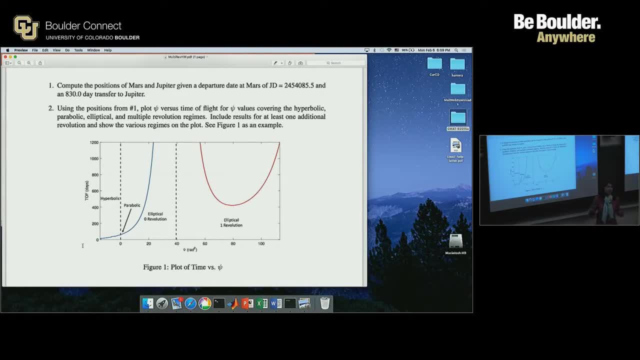 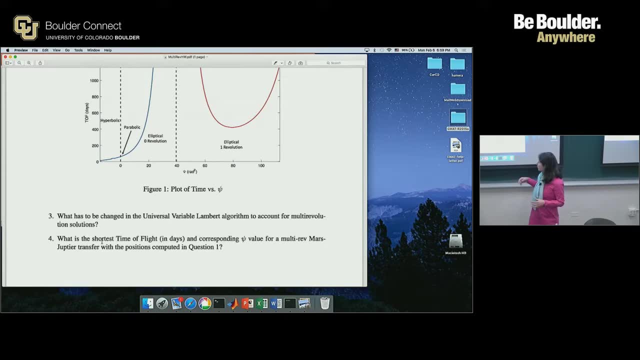 the one for Mars to Jupiter is going to look different, but it's going to have the same shape. And then we discussed this in class already, so hopefully this is a gimme. what has to be changed in your universal variable solver to get multi-rev? 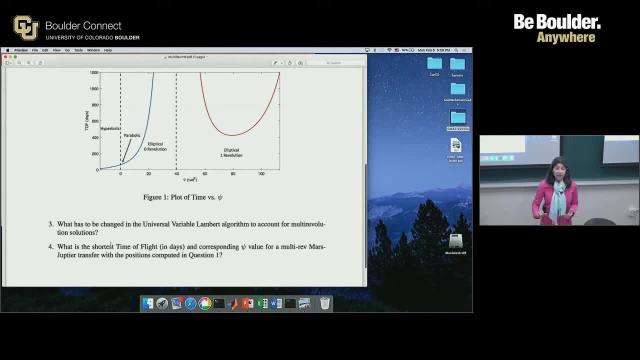 And then I want you to compute the shortest time of flight in days. So basically, that minimum on the red curve, The minimum time of flight that you need. Okay, Any questions on multi-rev? Okay, Okay, Then bear with me here. 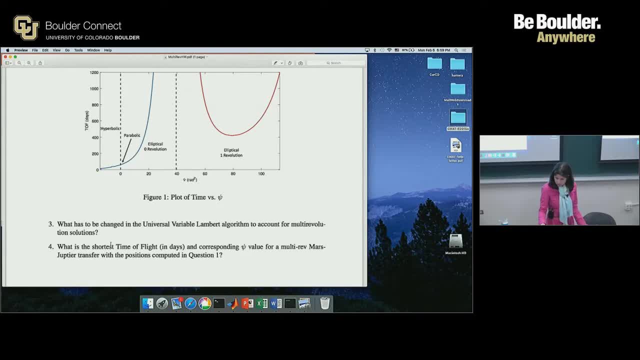 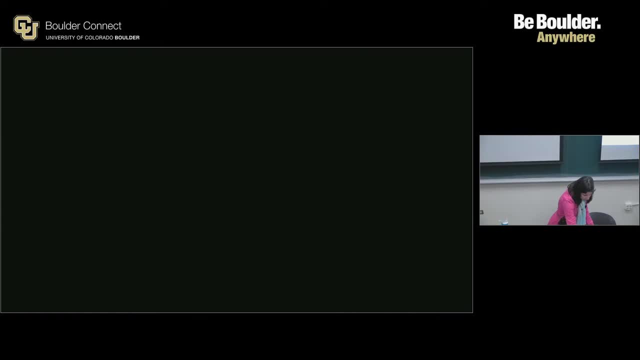 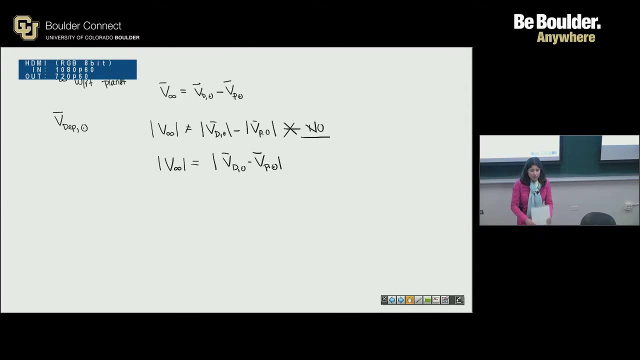 This will be the first time I've tried to give a lecture using this- the pen and the lectern- so hopefully it goes well. For the flyby, we're going to talk about gravity flybys now. And for gravity flybys: 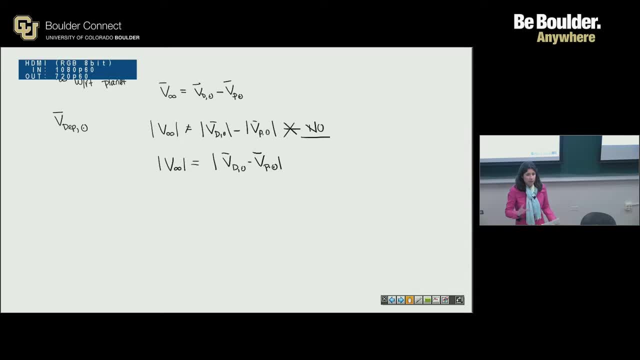 this is the kind of stuff I like to write out, because I think it's really helpful to have drawings at hand And to actually be able to draw it out yourself and see what's going on. So first I need my pen, Okay. 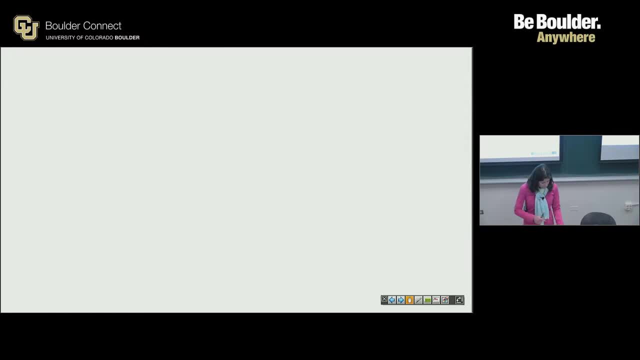 Let's go All right: Two, three, four, five, six, seven, eight, nine, 10,, 11,, 12,, 13,, 14,, 15,, 16,, 17,, 18,, 19,. 20,, 21,, 22,, 23,, 24,, 25,, 26,, 27,, 28,, 29,, 30,, 31,, 32,, 33,, 34,, 35,, 36,. 37,, 38,, 39,, 40,, 41,, 42,, 43,, 44,, 45,, 46,, 47,, 48,, 49,, 50,, 51,, 52,, 53,. 54,, 55,, 56,, 57,, 58,, 59,, 60,, 61,, 62,, 63,, 64,, 65,, 67,, 68,, 69,, 70,, 71,. 72,, 73,, 74,, 74,, 75,, 76,, 76,, 77,, 78,, 79,, 80,, 91,, 92,, 92,, 93,, 93,, 94,. 94,, 95,, 100,, 100,, 100,, 12,, 12,, 13,, 14,, 15,, 16,, 17,, 18,, 19,, 20,, 21,, 22,. 23,, 24,, 25,, 26,, 27,, 28,, 29,, 30,, 31,, 32,, 33,, 34,, 35,, 36,, 37,, 38,, 39,. 40,, 41,, 42,, 43,, 44,, 45,, 46,, 47,, 48,, 49,, 50,, 51,, 52,, 53,, 54,, 55,, 56,. 56,, 57,, 58,, 59,, 60,, 61,, 62,, 62,, 63,, 64,, 65,, 67,, 62,, 63,, 64,, 65,, 66,. 67,, 68,, 68,, 69,, 70,, 71,, 72,, 72,, 73,, 72,, 73,, 74,, 74,, 75,, 76,, 74,, 75,. 76,, 76,, 77,, 78,, 78,, 79,, 80,, 81,, 82,, 83,, 84,, 85,, 86,, 87,, 88,, 89,, 90,. 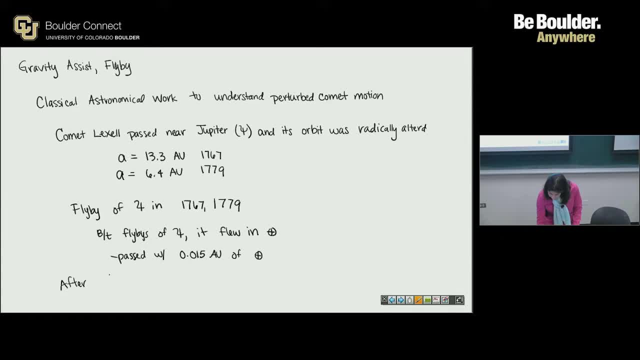 91,, 92,, 92,, 93,, 93,, 94,, 94,, 95,, 96,, 96,, 97,, 97,, 98,, 99,, 100,, 100,, 100,. 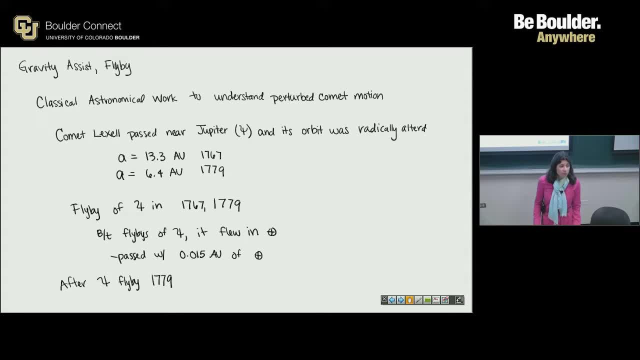 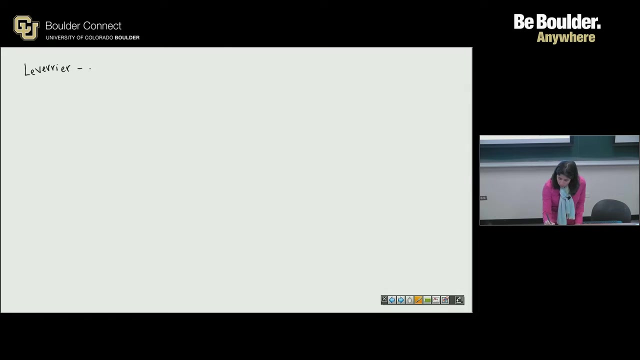 100, 100, 0, 100,, 100,, 100,, 100, 100.. H2logic alpha is to, to, to, to, to to, or time Laverrier. he realized that these orbits are modified by hyperbolic encounters. meaning: 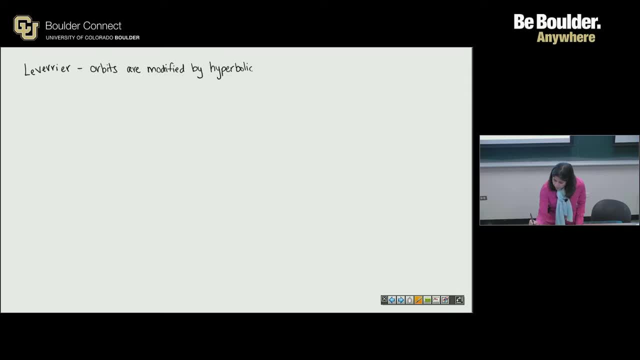 that while you're on a flyby, the spacecraft, the comet, whatever, as it flies by the planet, it's on a hyperbola with respect to that planet. It's not on an ellipse because it's obviously not getting captured by the planet. So you know it's on a hyperbolic orbit And he also. 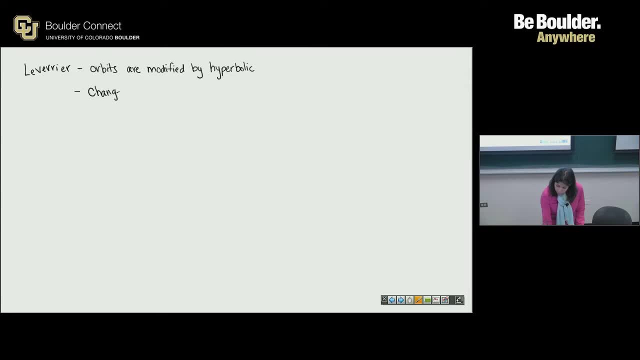 noted that it's changed, that after this gravitational flyby, that it's changed the orbital energy with respect to the sun. And that's really what we're looking for is changing our orbital energy with respect to the sun, Like if we want to get someplace more quickly or if we want to harness the gravity of other planets. we want to change our energy with respect to the sun. A man named Tisserand, I guess a little back story when they first, when they saw Comet Lexil those two times and one time it had really high semi-major axis. 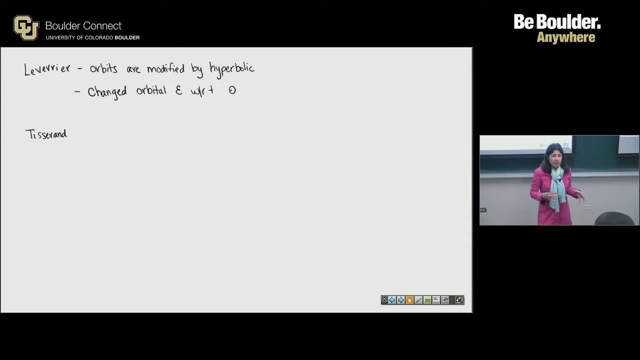 and the other time it had a much smaller semi-major axis. there was a controversy as to: well, how do we know? this is the same body that we're actually observing? Maybe it's something completely different. So, Tisserand, he came up with this criterion. 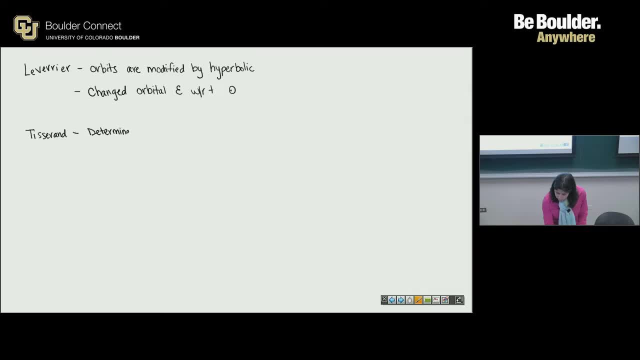 to determine if an observed body is the same as a previously observed body. So if you could take some measurements, you could see. well, is what we're going to do? is we're going to determine if what we just saw, is this the same asteroid we saw before, And he came? 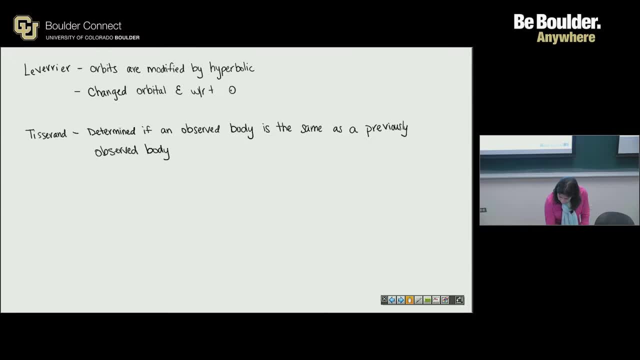 up with Tisserand's criterion. So he used the semi-major axis of the first, the eccentricity and the inclination, and he said: if you were to compute this quantity for the first, it should essentially be equal to this same quantity for the second, Or in other words, 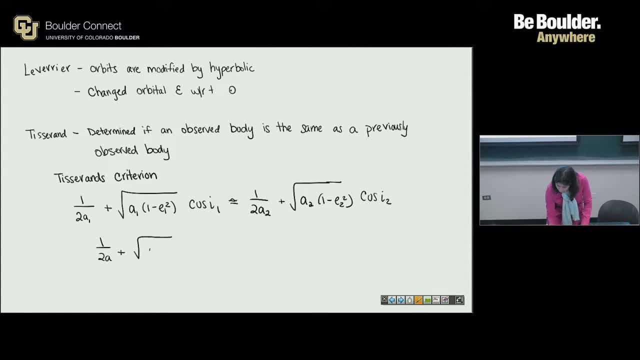 this one over two, a plus the square root of a, one minus b squared, So that means that the cosine of the inclination is approximately constant. So then they were able to determine. you know, was that these comets were the same. OK, Between 1920 and. 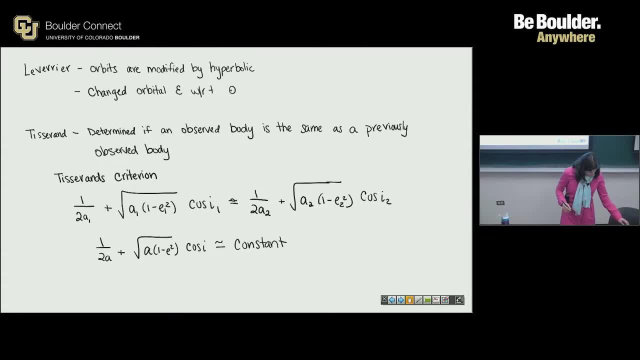 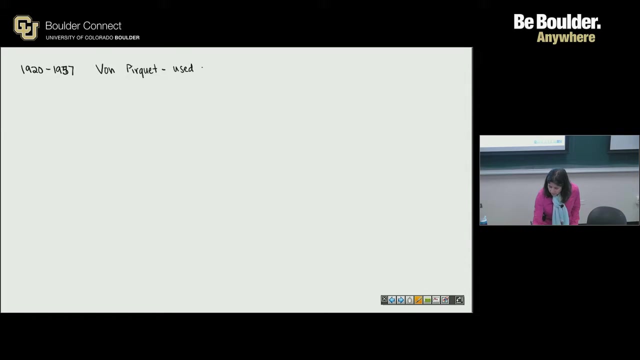 1957, let's see, OK, so that was kind of the classical astronomy in the 1700s and the 1800s, In the 1900s, so let's say 1920 to 1957, a man named Von Perquet- he used vector diagrams which 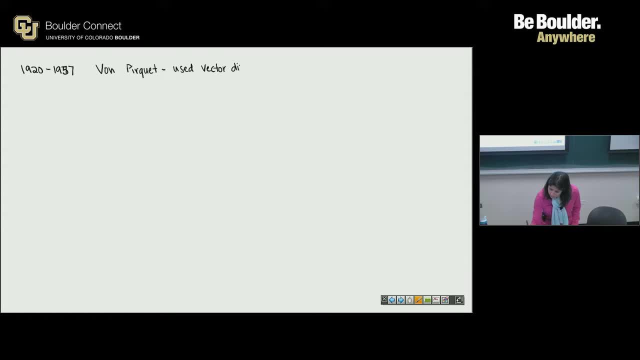 will hopefully become your friend- to model flybys and to show modified energy. XXX, CE II, XXX ущ. around this time there were also a lot of science fiction writers and they kind of- you know, in a qualitative sense understood what was going on. The science fiction writers were using flybys in their solar system exploration. They might not have had you know, all the physics entirely right, but there were a lot of stories out there where these brave explorers were using gravitational flybys to get to distance. 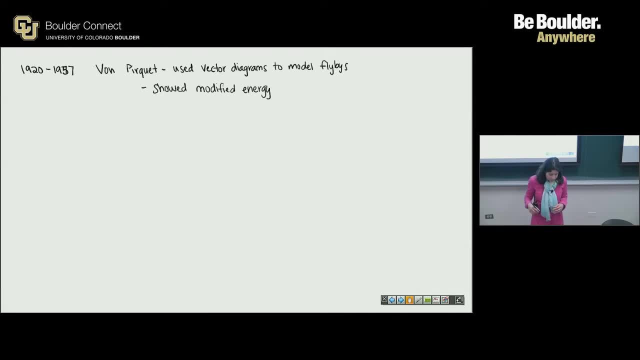 Glu death R? U dites s earth" or planets or whatever. And then you know, basically, since 1958, we've been, there's been applications of flybys. So the basic idea of a flyby is to alter. 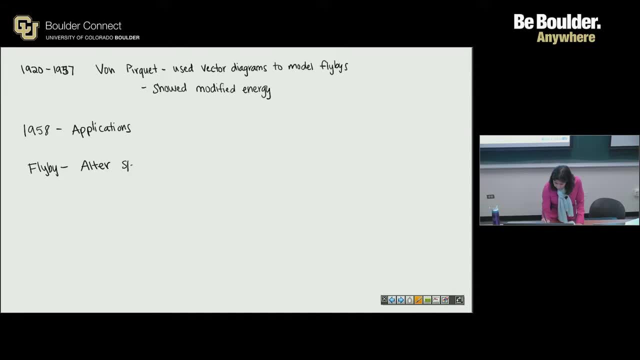 the spacecraft's energy with respect to the Sun. So we're also essentially getting what we'll call free energy Flybys, as we saw. in the very first lecture I talked about Ulysses. Anyone remember what Ulysses did? Fly by the Sun. 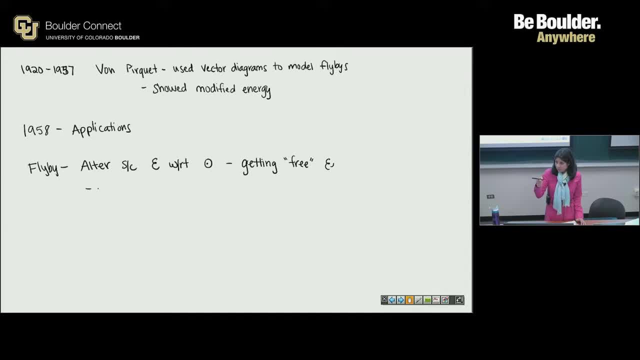 It flew by Jupiter to get to the Sun, Yeah, to get into a polar orbit about the Sun. So you can use flybys to change inclination. So we'll just see Ulysses' mission. Okay, one thing that we do need: 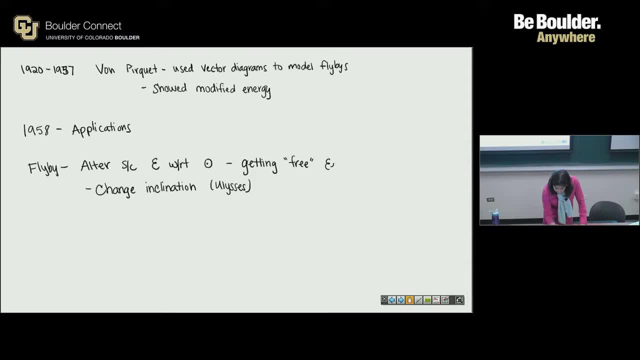 to note about flybys is that angular momentum is conserved. Okay, so let's just say that we are flying by a planet and the spacecraft's energy with respect to the Sun is going up. So what's that going to mean? for if? 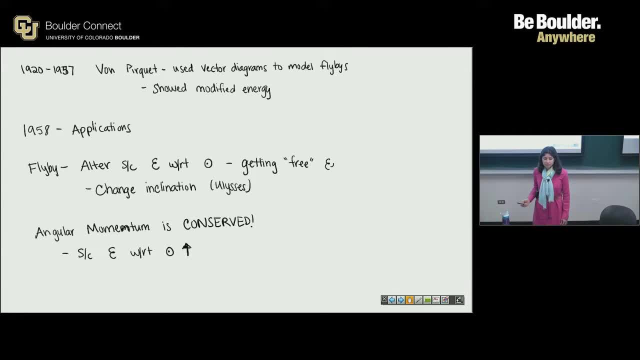 our angular momentum is conserved, The planet you're going about is losing energy. Yeah, Yeah, So the planet's energy with respect to the Sun is going down. So if the spacecraft's energy with respect to the Sun decreases, then the planet's energy will increase. 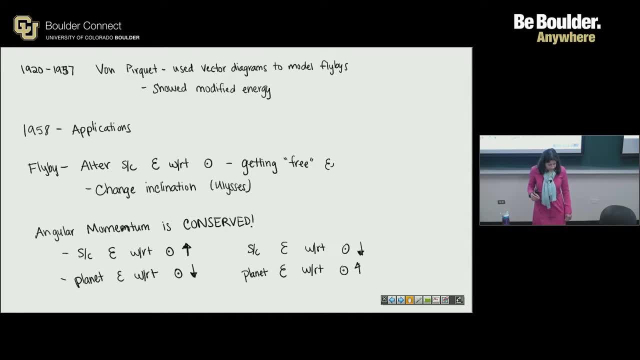 Okay, Now are we worried about, Yeah, the energy change of the planet. Like is sending spacecraft, you know, doing multiple flybys of the planets, just going to throw the planets into chaos because they're losing energy? Like, are we dooming the solar system by what we're doing here? 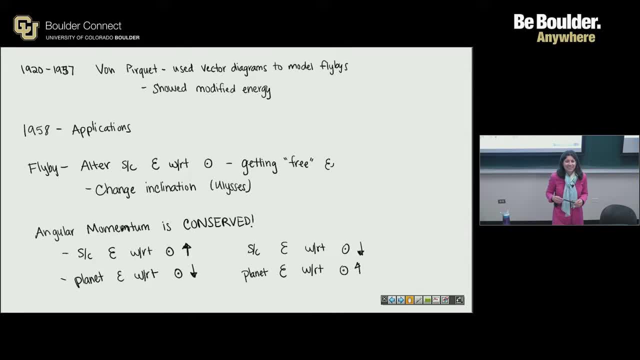 If we had the Death Star, maybe. Huh, If we had the Death Star, maybe, Maybe. if we had the Death Star, That would be awesome. That would be a really interesting physics problem. I'm just thinking about this in my head now, like 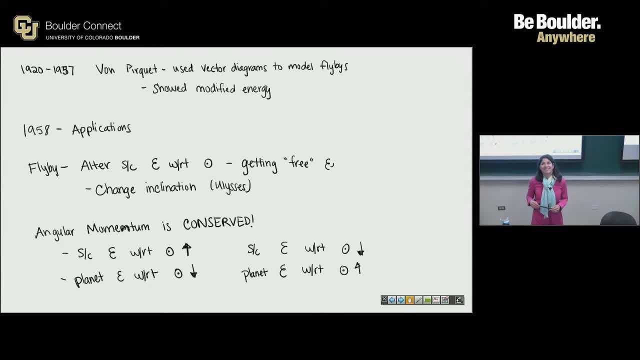 Okay, Rather than blowing up planets, we're just going to send them on. We're just going to eject them from the solar system. Okay, So are we worried about our spacecraft doing that? No, we're not. We are not worried. so 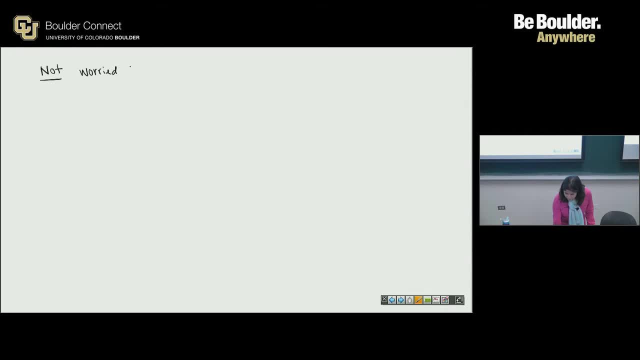 Not worried about the energy change. Why is that Mass is negligible. Yeah, Yep, The mass of the spacecraft is much, much less than the mass of the planet. It's essentially negligible. Okay, So let's talk about what actually happens inside the sphere of influence. So what happens? 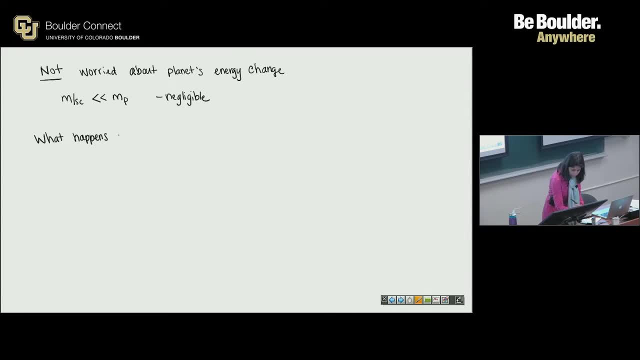 inside the sphere of influence. Okay, So inside the sphere of influence, the spacecraft enters- this is important to understand- it enters and leaves the planet's sphere of influence with the same energy, The same energy relative to the planet. Okay. 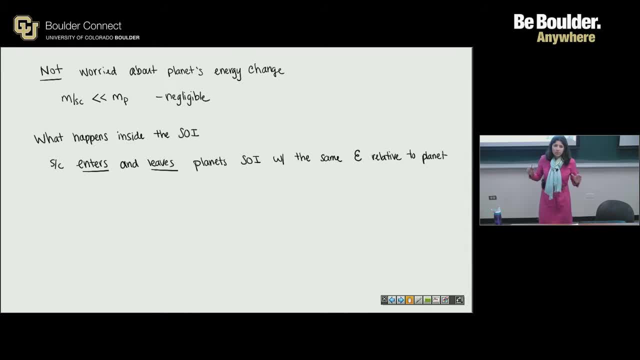 So, relative to the planet, as the spacecraft comes in on this hyperbolic trajectory, it's the same hyperbola as you enter and leave, right, So no energy change. Okay, The flyby is hyperbolic, So we can say that at infinity, let's just use the energy equation: Energy at infinity. 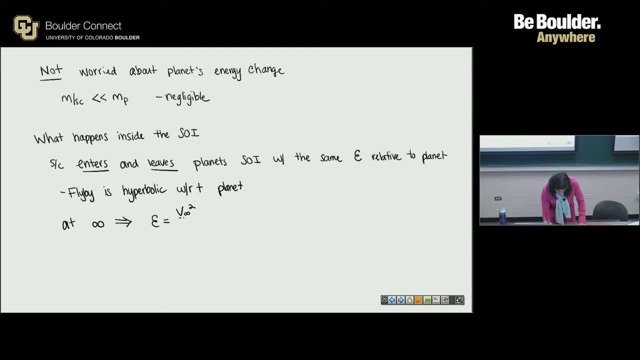 is going to be the infinity squared over 2 minus mu over r is minus mu over 2a. Well, we cannot. We can kind of say that this is r infinity, right? So what's going to happen to that term? 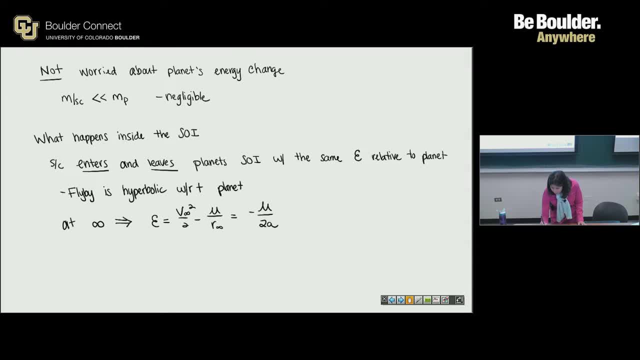 Yeah, this term essentially goes to zero, because r is infinity. Now again, we're just making an approximation. that's not entirely true, but we can say that energy is now v infinity squared over 2.. So, just to let you know, I'm going to use the notation plus to be outgoing at the flyby. 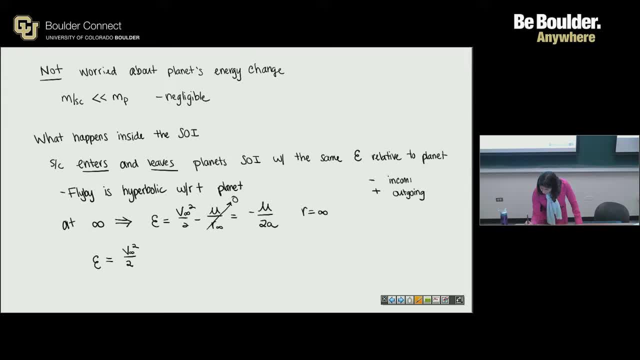 and a minus sign to be incoming at the flyby. So we can say that energy coming into the flyby is v infinity coming in squared over 2.. Energy coming out is also v infinity squared over 2.. So we have, since we don't have any energy change v infinity in is equal to v infinity. 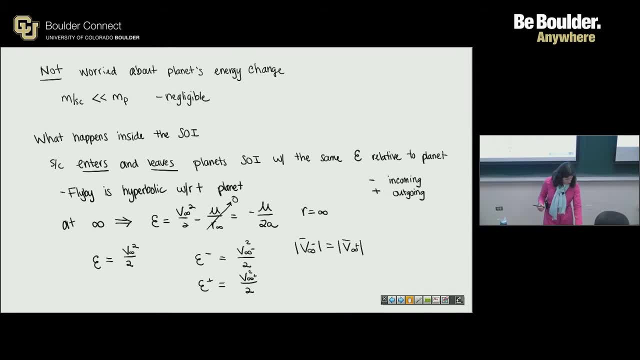 out. Okay, Everyone, have all this. before I go to the next slide, I'll just give you a minute. Now again, I'll just put: assumes no perturbations. How are we doing on time? Good, So for our preliminary mission design, assuming no perturbations is a good approximation. 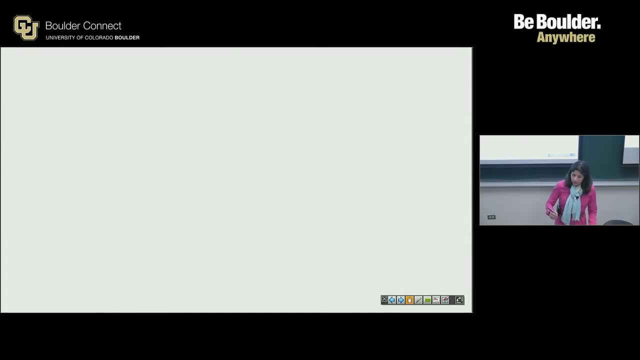 Okay, So we've said that v infinity in In equals v infinity out. Sometimes people will, you know, say in and out. but does that mean that? Is that statement true? No, This statement is not true, because we're changing directions. 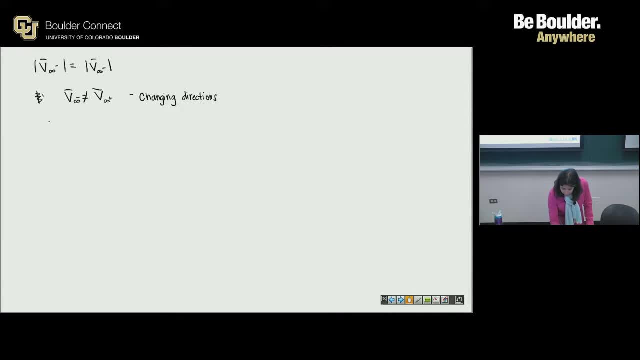 Our flyby vector is turned. So that is not true. The magnitudes are the same, but the velocities are different, So components of velocity are different. Okay, So let's just look at a vector diagram here. Here's our planet and here's the velocity of the planet. 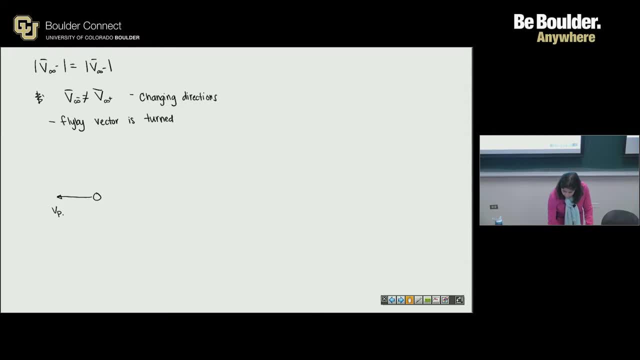 All right. So let's just say we've got this nice hyperbolic trajectory, We've got v infinity in and v infinity out, So let's draw a vector diagram for the flyby. So So we'll start at. 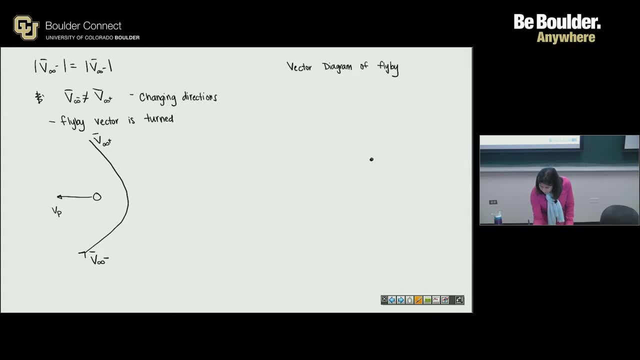 I'll just, I'll just put the sun here. So here is the velocity of the planet, and that's with respect to the sun. Okay, Now v infinity in and out are with respect to what The planet, Okay. 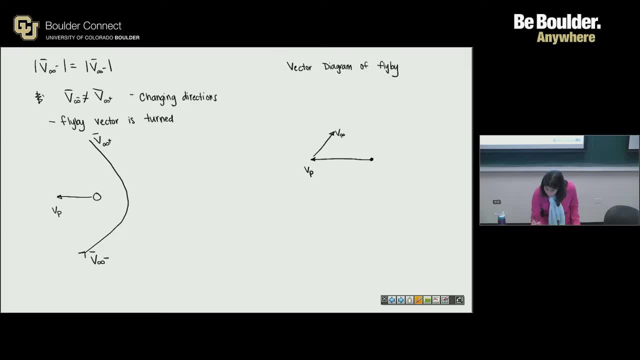 So let's just draw. Here's. It kind of looks like it's going in that direction. There's v infinity in And here's v infinity out. Okay So, and I tried to draw those the same length because they're the same magnitude. 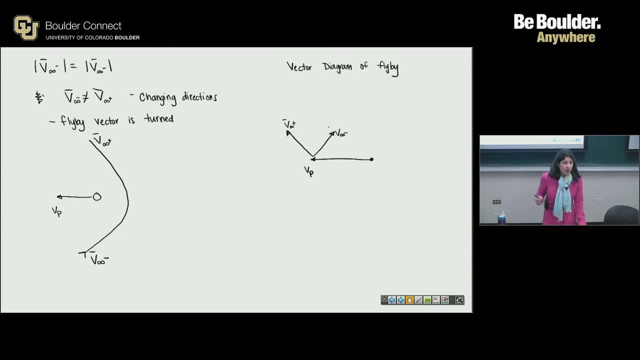 Right, So from our Lambert solver we have our departure and arrival velocities with respect to the sun. Okay, So here we've got. This would be v arrival at the planet. So that's the hyperbolic, Or, sorry, the heliocentric velocity, as you're coming in on your conic orbit. 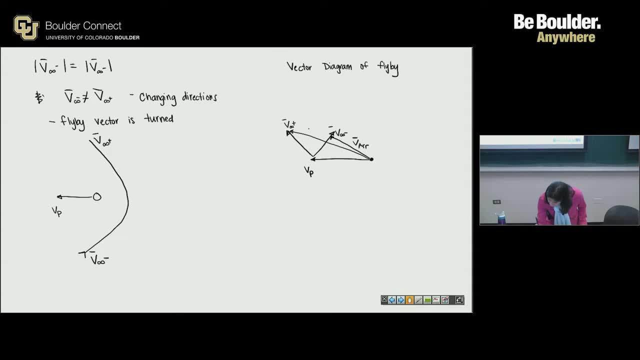 And then here is the departure velocity with respect to the sun: Okay, So v arrival, It's the velocity on a heliocentric orbit, So that's the transfer orbit that you would get from Lambert's. Okay, And velocity at departure is the velocity 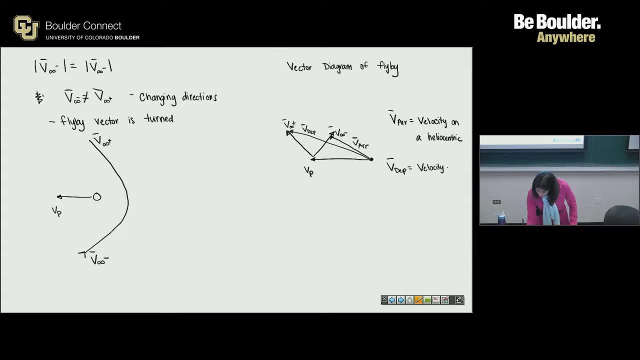 Oh, not arrival, sorry, This is on a heliocentric orbit at departure, Okay, So sometimes we'll just call. We could also say that this is the spacecraft's velocity with respect to the sun at departure, And this would be. 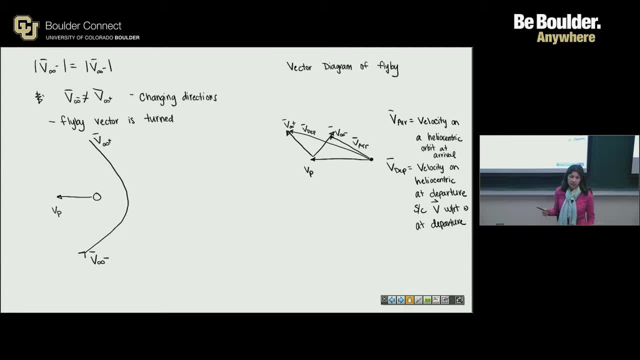 V arrival would be the spacecraft's velocity with respect to the sun at arrival. And so now hopefully it's really clear that you can see That v infinity incoming is just the velocity at arrival minus the velocity of the planet, And v infinity outgoing is the velocity at departure minus the velocity at the planet. 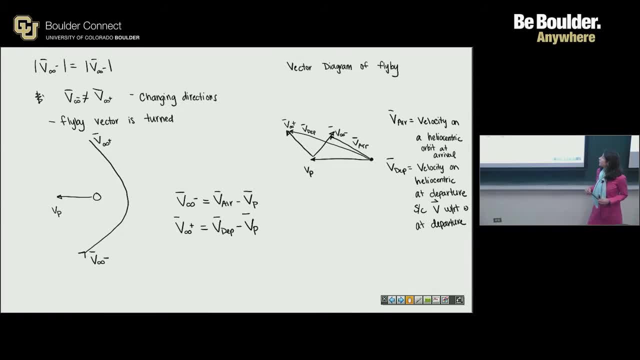 And so now, what can you see about the two departure and arrival velocity vectors? At least magnitude-wise, Departure's bigger, Yeah. So just looking qualitatively, we've really increased the magnitude of our departure velocity by this flyby. 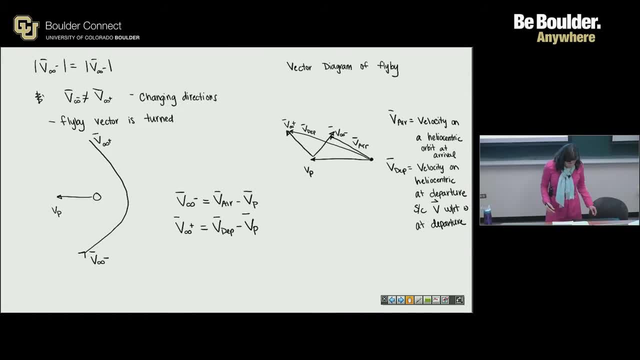 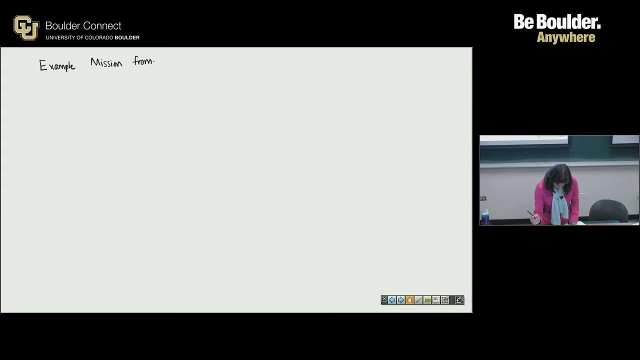 Okay. So let's just kind of talk through. Does everyone have this? Okay, Let's talk through how we're going to get all these velocities. So let's just do. Let's do an example mission from: Let's go Earth to Jupiter with a Mars flyby. 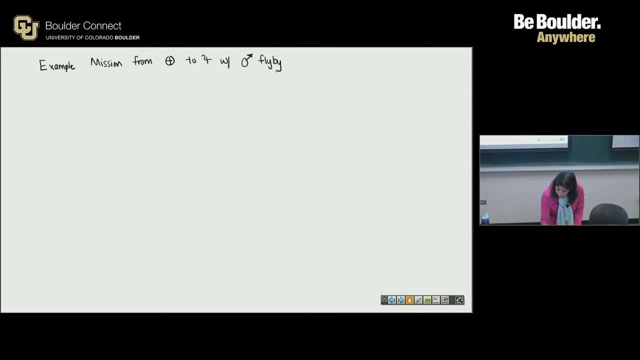 Okay, So essentially Earth to Mars, to Jupiter. So how are we going to? So we're flying by Mars. How do we find all these velocities? So for the flyby we need v infinity in, v infinity out, velocity at arrival and velocity 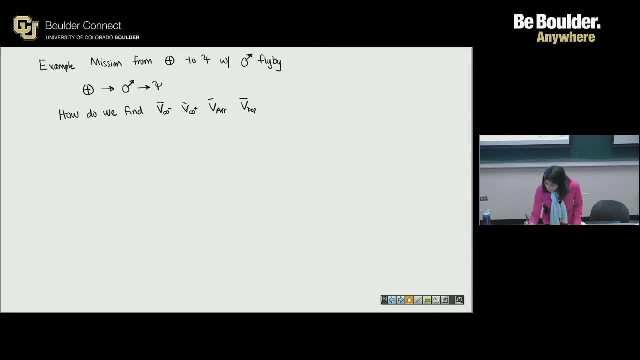 at departure at Mars. So how do we find all those things? So what can we find? Let's say we're given the dates. Let's just say we're given the dates of the events, So we know Earth launch, Mars flyby and Jupiter arrival dates. 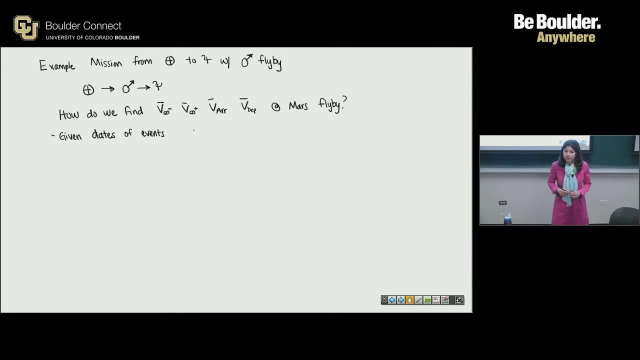 What can we do? Velocity of the planets: Okay, We can get the velocity of the planets. So we can get the velocity of Earth, velocity of Mars and the velocity of Jupiter. What else can we get? Lambert gives the arrival velocity. 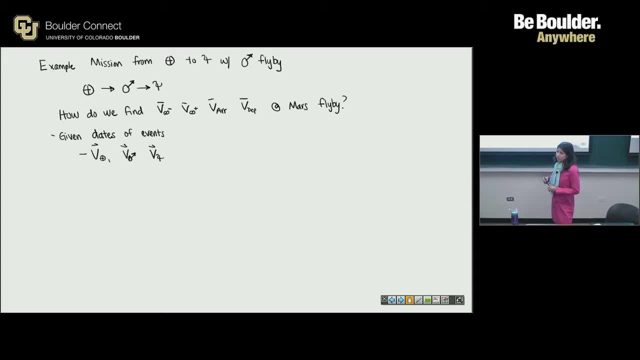 Yeah. So how do we get the arrival velocity? Where would we solve Lambert's? Okay, Where would we solve Lambert's? Which two would we use? We want the arrival velocity at Mars. What are we putting into our Lambert solver? 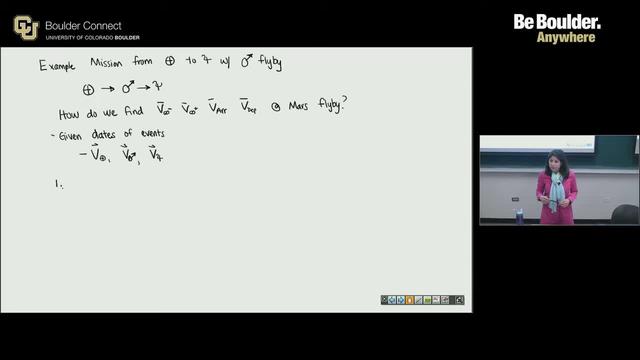 Position of Mars And Earth. Yeah, So we'll solve Lambert's From Earth to Mars. This will give us our velocity of arrival at Mars. All right, So from the arrival at Mars, then we can get our incoming the infinity. 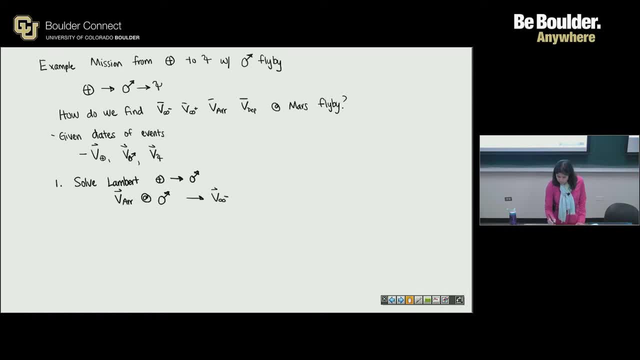 Because we've got our velocity at Mars and we've got the velocity of Mars itself. Okay, So what about our departure velocity From Earth Or from Mars? From Mars, If we're going to, What's the departure velocity out of Mars? 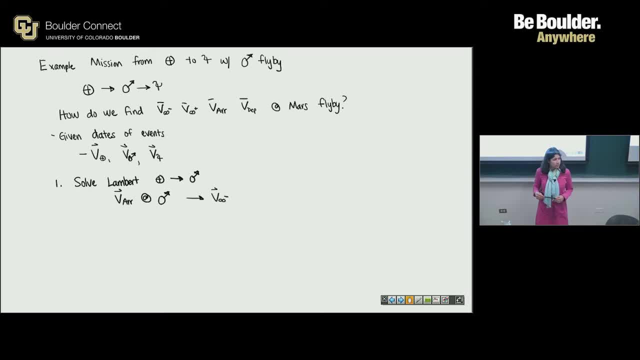 How could we get that Vector diagram? We could maybe do a vector diagram. Let's think about that. So if we wanted to do a vector diagram, we Right now we've got V infinity at Mars and V infinityor. we only have V infinity at Mars and we only have our arrival velocity at Mars. 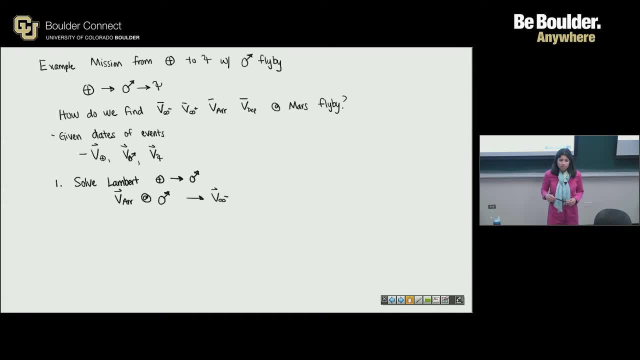 You need to know how close you're going to get to Mars, right? How could we solve for that Turning angle? Well, if we don't have V infinity out, we know the magnitude of V infinity out, but we don't know the components. 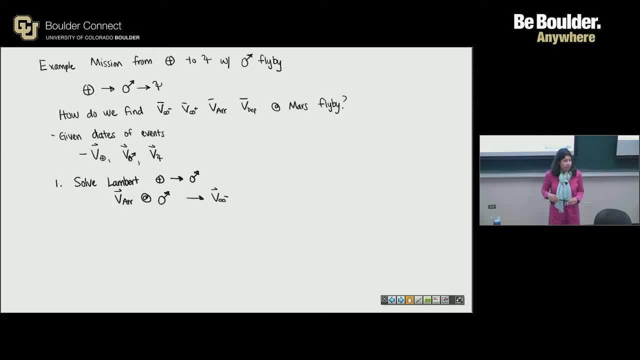 So if we don't know the components then we can't get a turn angle. We can solve Lambert's problem for Mars, Jupiter. Yes, We can solve Lambert from Mars to Jupiter And then that will give us our velocity departure at Mars and so we can get V infinity outgoing. 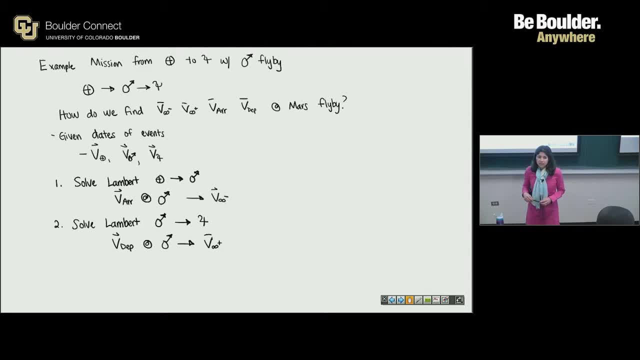 Okay, So now we've gotnow. we've got our flybys Now. In the diagram I drew before we showed kind of our departure velocity looked larger than our arrival velocity. So we've essentially got two ways to fly by the planet. 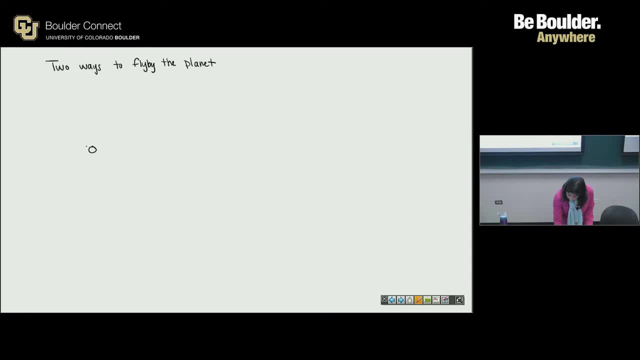 So ifthis is our planet, here We've got the velocity of the planet. We can fly by like this, where we've got V infinity in, V infinity out, Or we can fly by like this where we've got. 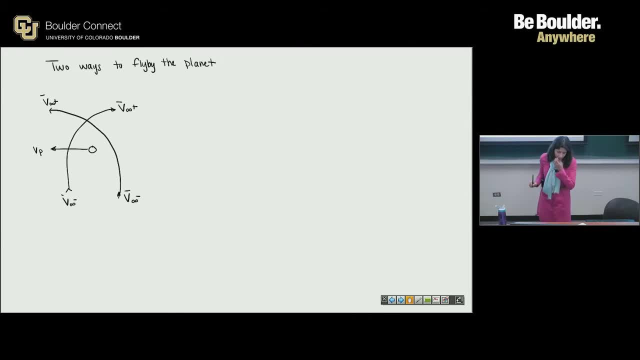 and V infinity out, All right. So I'd like you guys to work together. Not work together, but you know, in groups by yourselves. Just do a little in-class exercise. I'd like you to draw the vector diagrams for both of these cases. 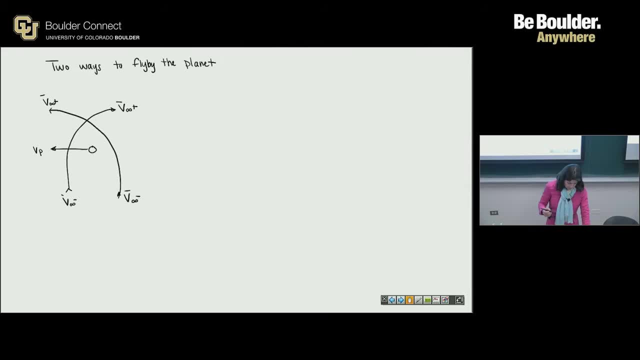 And look at energy changes. We'll call this a pass-ahead, Or a leading Pass-ahead And a pass-behind over here. Okay, I'll give you guys a few minutes. Draw the vector diagrams. velocity of the planet. 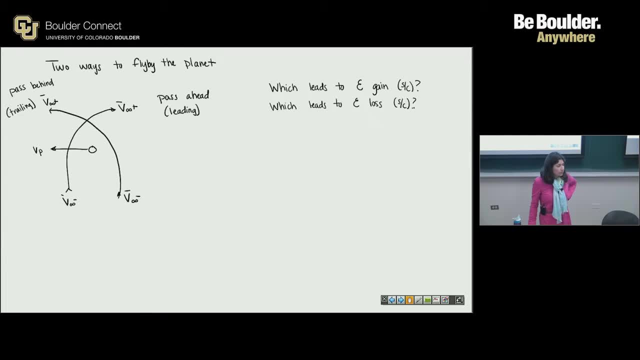 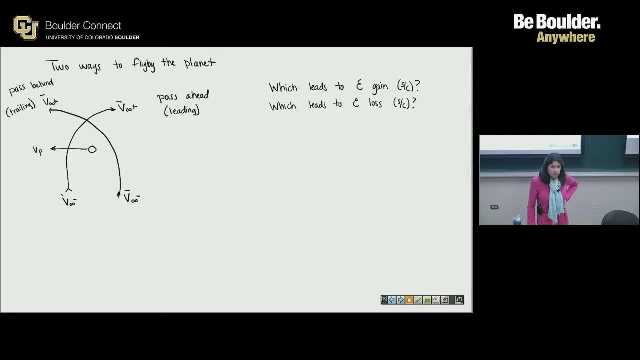 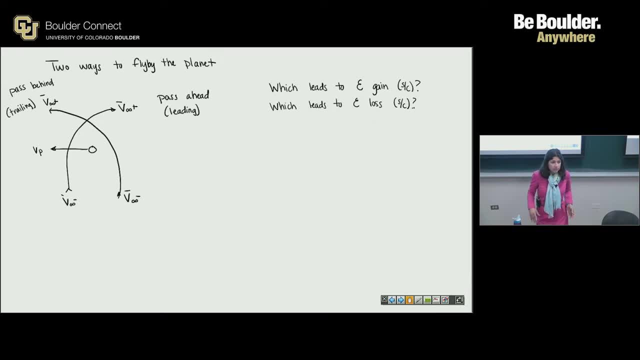 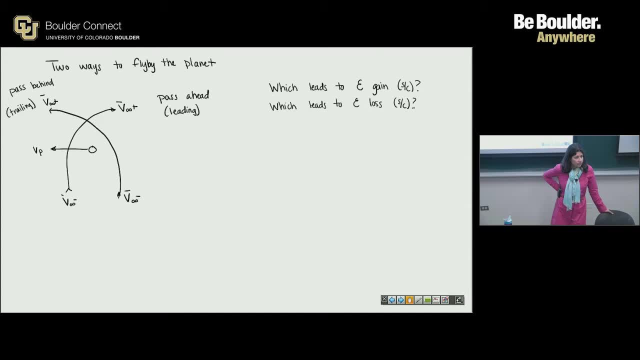 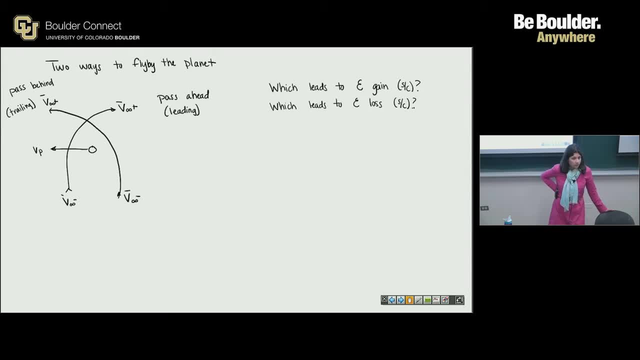 7, 6, 7, 8, 8, 9, 9, 10, 11, 12, 13, 12, 13, 13, 14, 15, 16, 17, 18. Okay, so which of these flybys? the pass ahead, or the leading, or the trailing? flyby is going to lead to an energy gain. If we want to gain energy, which way do you want to fly by the planet, Behind the planet? And if we want to lose energy, Yep, so I'll just draw them real quickly. Let's just say that we're 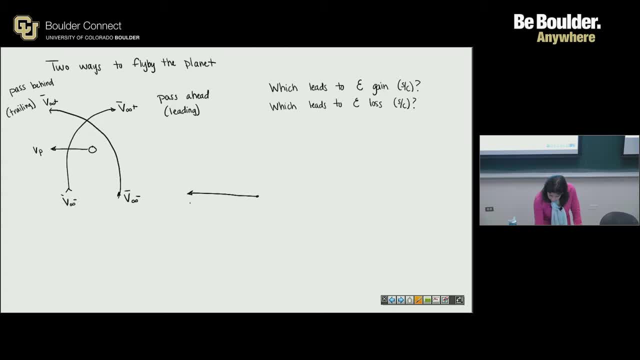 let's just do the behind case. So here's the velocity of the planet. I tried to make this like vector diagram, somewhat easy. So here's V infinity minus V infinity plus going this way. So here's our velocity at arrival and our velocity. 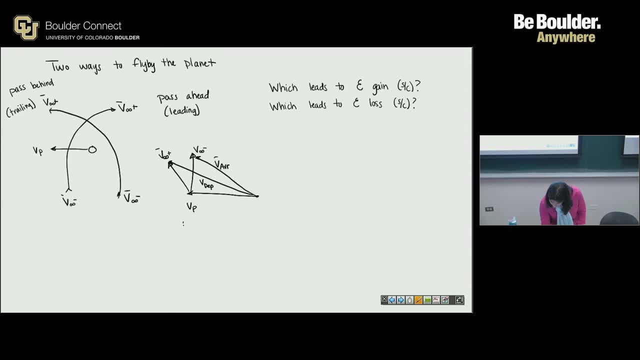 at departure. So here we've got trailing And we've got an energy gain, Because the magnitude of the departure is going to be greater than the magnitude of the arrival. If we look at the leading case again, the velocity of the planet here's V infinity. 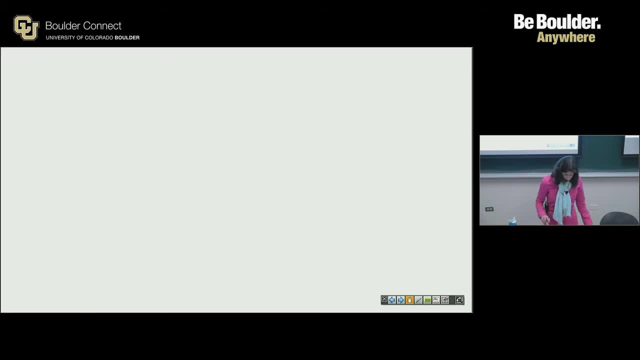 incoming. Aha, okay, But now V, infinity out is this direction. So velocity at departure is smaller than velocity at arrival. So for the leading, we have trying not to like, bump it with my hand here- energy loss And our velocity at 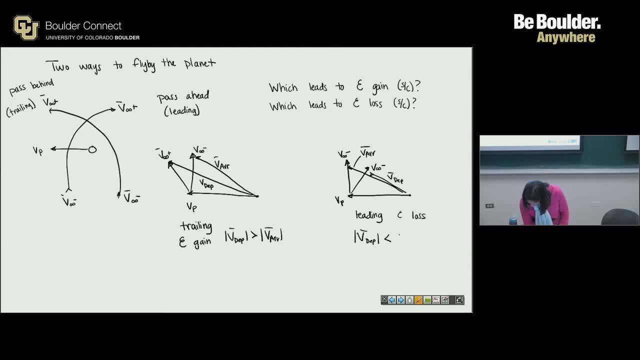 departure is less than our velocity at arrival. When might we want a leading or trailing flyby? Let's talk about the leading flight flyby. Why might we want that? Trying to get to planets that are closer to the sun? Yeah, get to planets that are closer to the sun. 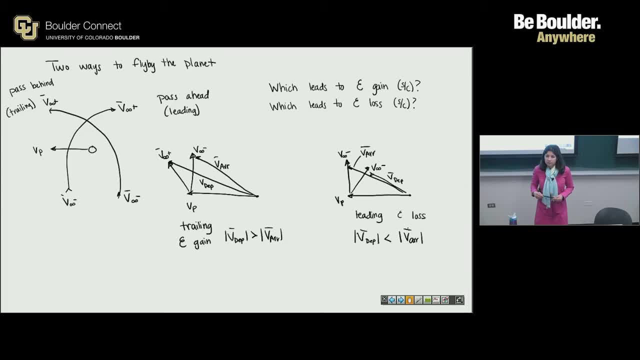 If you want to try and slow down, essentially And obviously the converse is going to be true for going out- All right. so now we've got our, we've got a way to get the incoming velocity and the outgoing velocity with respect to the 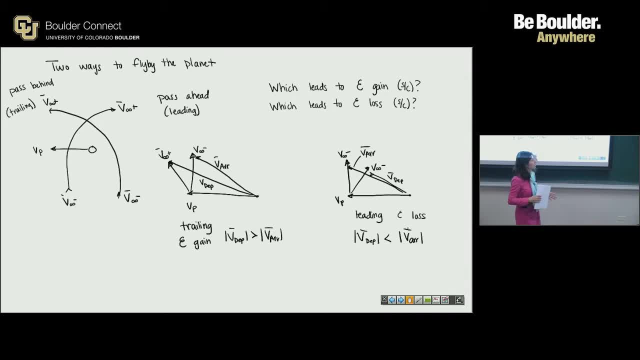 sun. We can figure out our velocity, our hyperbolic velocities, with respect to the sun. Now we need something very important when doing a flyby Anybody. What's very important when doing a flyby? Yeah, you don't want to hit the planet. 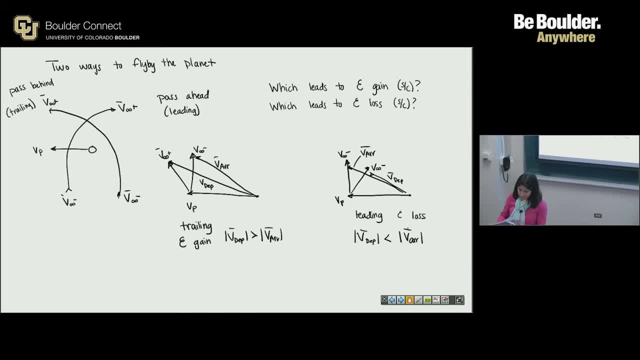 So let's talk about how to get the radius with respect to the planet. So for that I'm going to provide nice little hyperbolas to draw on, because I think it's just nicer that way, And we're going to try this guy here. 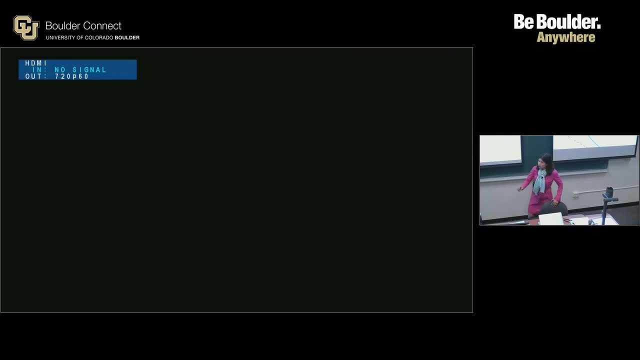 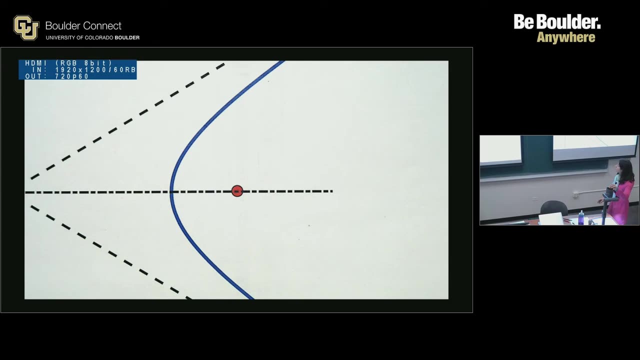 Hopefully we'll try this. Oh Okay, Zoom out Gears. It's kinda nice not to get chalk dust all over my hands. I mean it's not so bad. You only do this with the other extracts. Do anyone have any questions? I'll put the. hand up so I can keep them to myself. Now it's time to take it until I get players to their favorite planets. 5-12 Tu 의 Space Space Boom 1-o. Space Space Boom for the city, since the incident two days away from a. 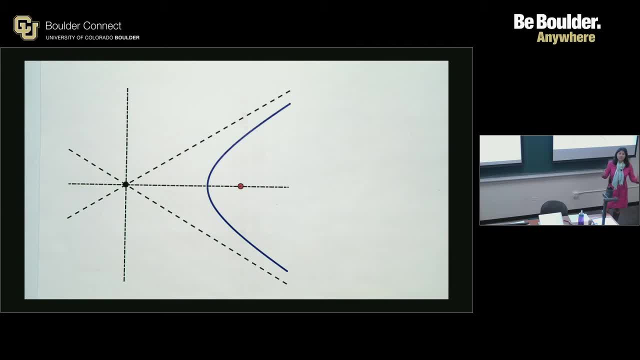 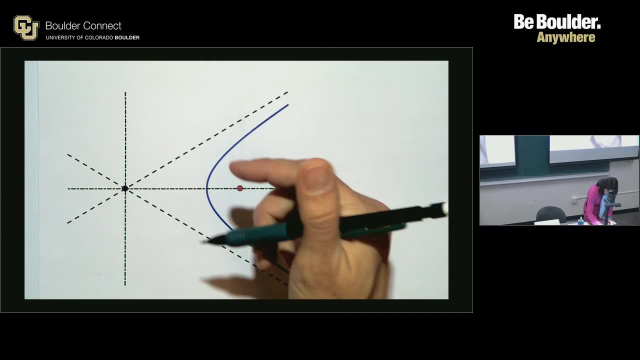 on those vector diagrams. Does that all make sense, just from a nice geometric point of view? Okay, good, All right. so first let's just start by labeling some parts of the hyperbola. So if we're looking at this distance right here, 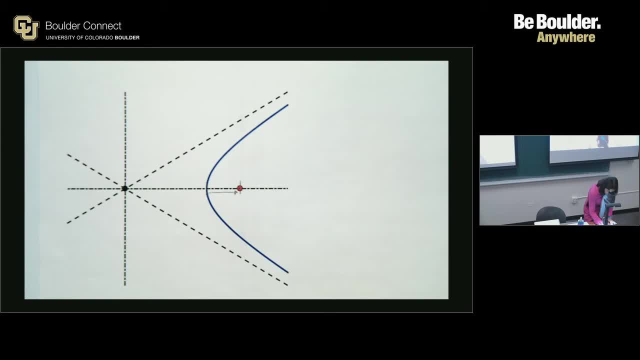 anybody Periopsis, so we'll just call that r sub p. That's what we want to find out. How do we get r sub p so we don't crash into the planet? Okay, this value here if we were to drop a perpendicular line. 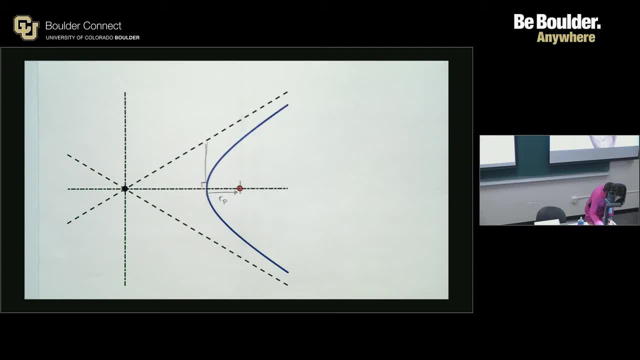 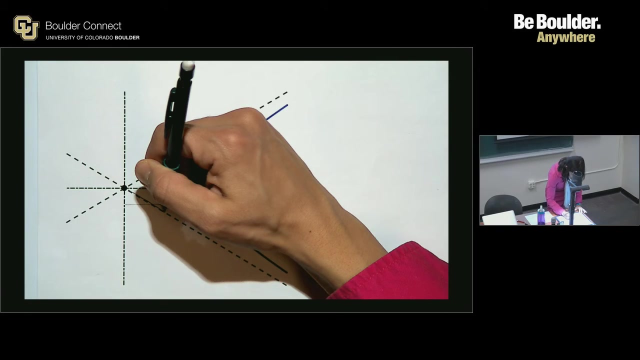 right at periopsis. this value is b, the semi-minor axis, And then this value is the semi-major axis And this tangent line right here. if we've got a and b, anybody have any brilliant guesses as to what this tangent line is? 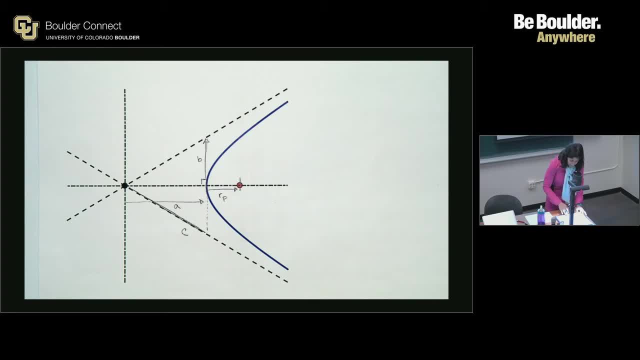 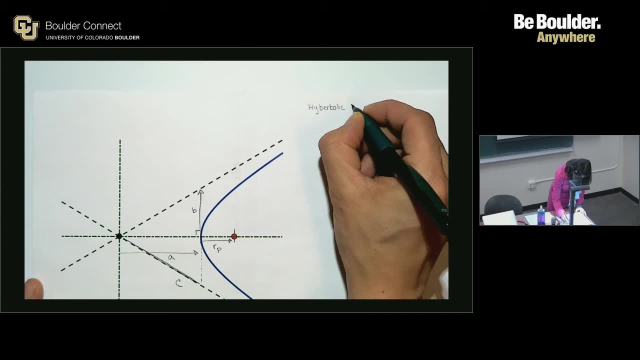 C. All right. so for the hyperbolic equations, c Gosh, The general equation for a hyperbola is: x-squared over a-squared minus y-squared over b-squared equals 1, where c-squared is a-squared plus b-squared. 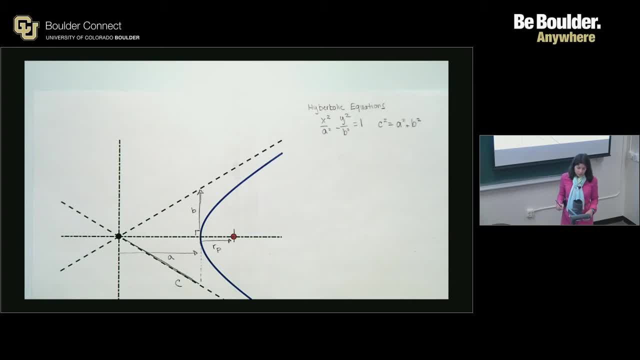 One thing to note for hyperbolas, just by definition, is that the semi-major axis is what? positive or negative? Negative. So we'll say that r sub p. we can define that as a minus c, but we have to note that both a and c. 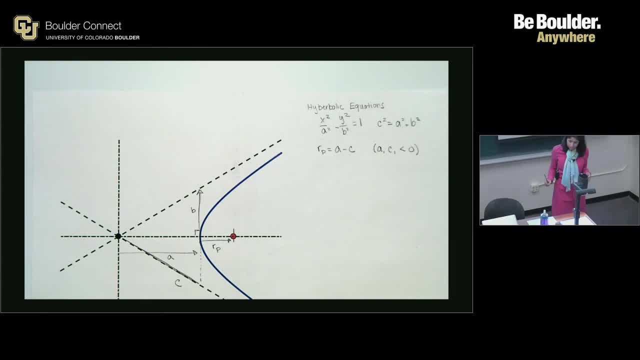 are less than zero for a hyperbola. So let's just define it this way: where we've got our incoming b-infinity vector and our outgoing b-infinity vector, All right. so now we're going to start looking at the turn angles. 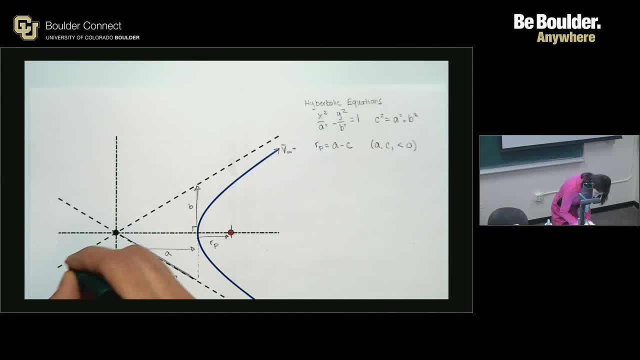 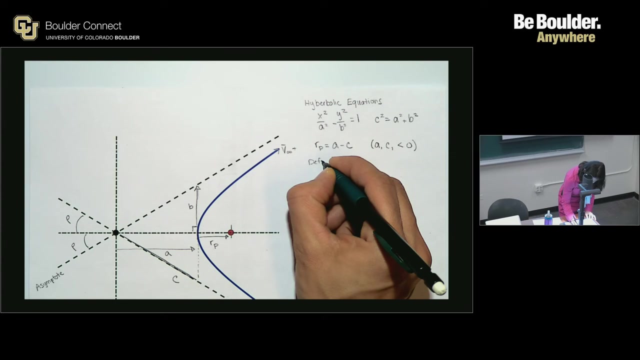 Obviously, these dashed lines are the asymptotes of the hyperbola And if we define an angle between the line from the origin, through periapsis, and the asymptote, we'll call it rho. So these values are rho and we'll define rho as the asymptote half angle. 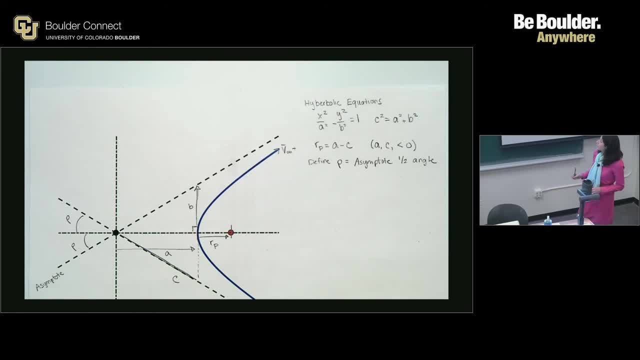 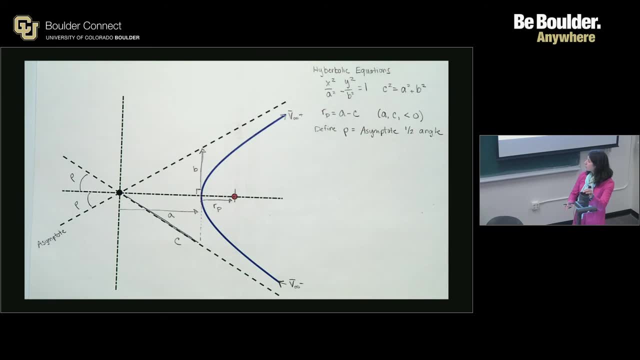 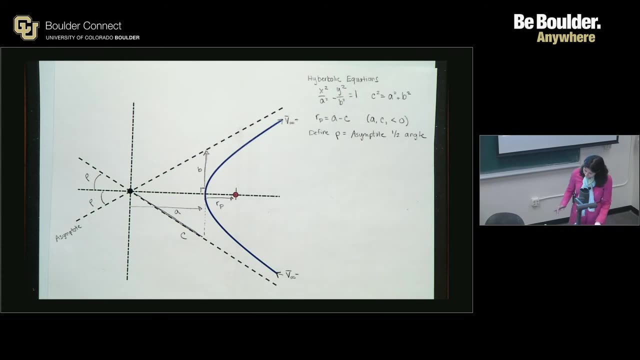 Oh, sorry, this is sliding down a little bit. Let me zoom out just a smidge. If you can't see something, just let me know. Hopefully we can. oh, I'll probably okay. Now we're also going to define so the angle through which v-infinity in is turned. 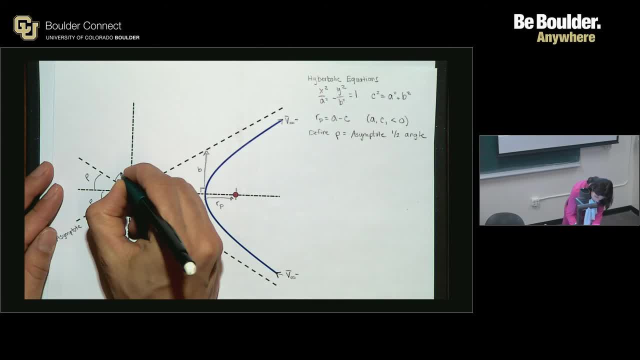 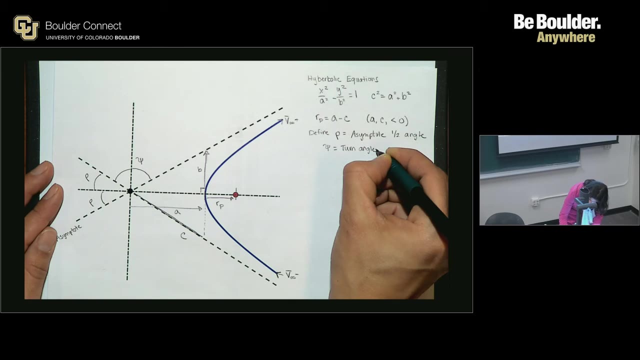 to v-infinity out. we'll call the turn angle psi. I know that's confusing. this is different than psi of Lambert's. okay, So psi is the turn angle and it's different than Lambert's. So conveniently we can write a relationship between psi. 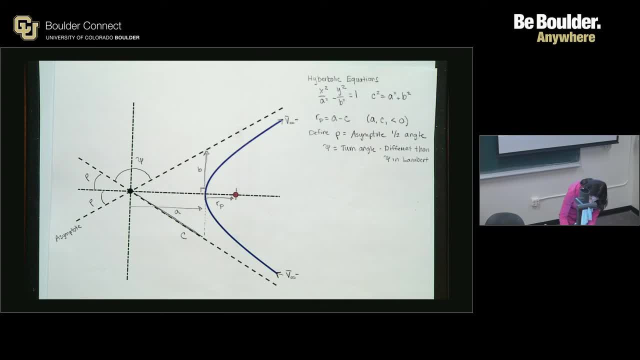 and rho. what would that be? Psi is Yeah, pi minus two rho. All right, Now we want to eventually get the radius of periapsis, and we have the radius of periapsis as a over c, So let's see if we can work with that. 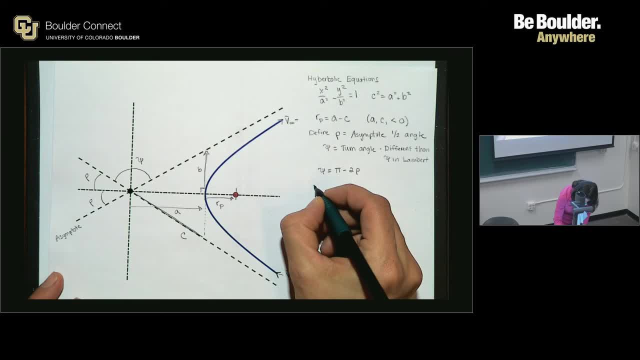 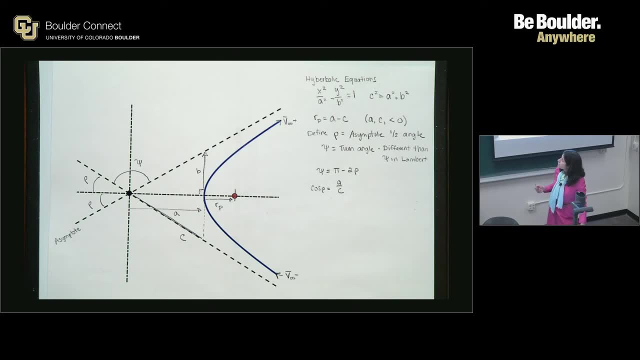 So we can define: the cosine: of rho is a over c, And we've already said that r sub p is a minus c. So let's make some substitutions here. So we'll do. we can now make one over c, over a. 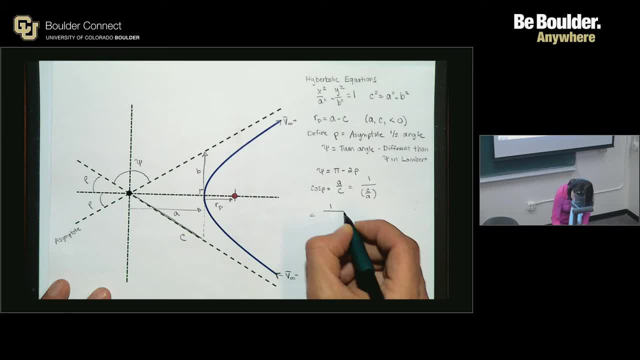 and then do one over a minus. we'll do a minus c over a. So now we've got something in terms of the semi-major axis and the radius of periapsis. Okay, Okay, We're going to multiply by mu over mu. 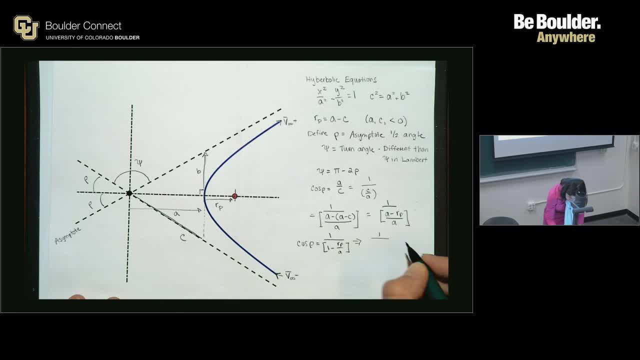 and rearrange. So we'll have one over one minus. we'll take mu over a times r, sub p over mu. So basically I just multiplied by mu over mu and rearranged this. So now we can take a look at the energy. 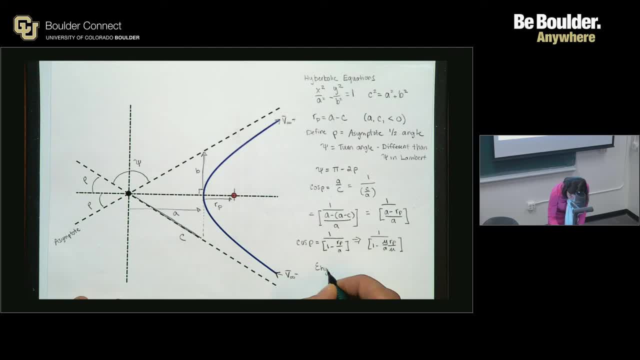 The energy of a hyperbola is just v squared over two. And then, remember I said, minus mu over r goes to zero, because we are looking at infinity. And this is also equal to minus mu over a. Two a, That's right. 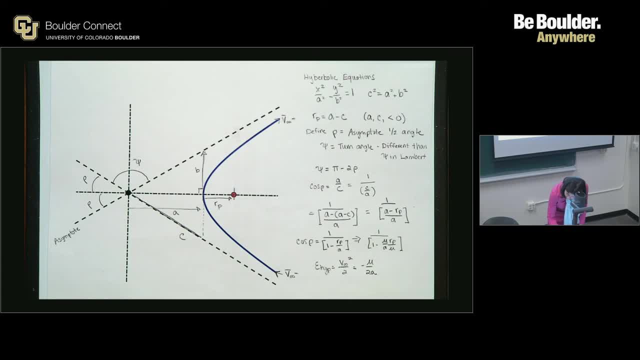 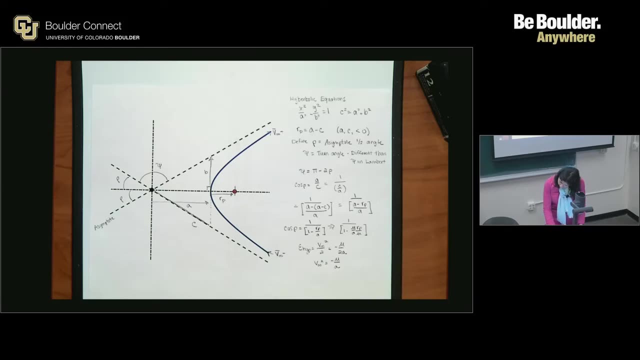 So if we were to rearrange this, we can basically just say that v infinity squared is minus mu over a. All right, let me zoom out. Okay. Yeah, we have time. Okay, So let's substitute this equation back in here. 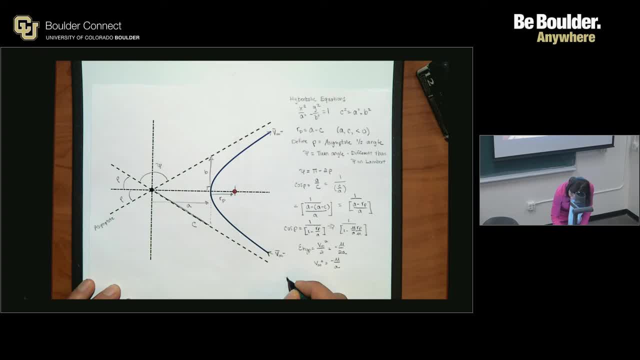 So we'll have cosine rho is one over one plus b infinity r sub p over mu. Okay, And if we can recall, we have a sine of one over one plus b infinity r sub p over mu, So we can substitute that back in. 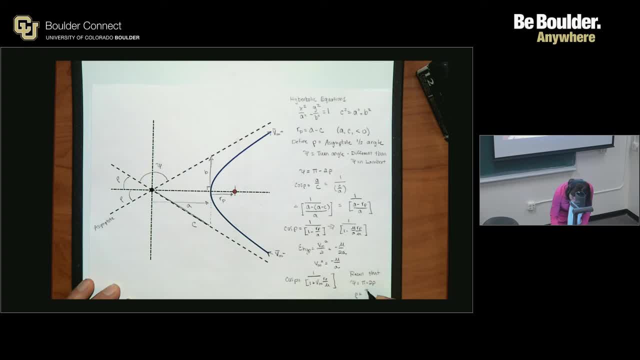 So we'll have: rho is pi minus psi over two. Let's pull this out over here. Let's just kind of rearrange this. We'll have one plus v infinity. r sub p over mu is equal to one over or cosine of rho. 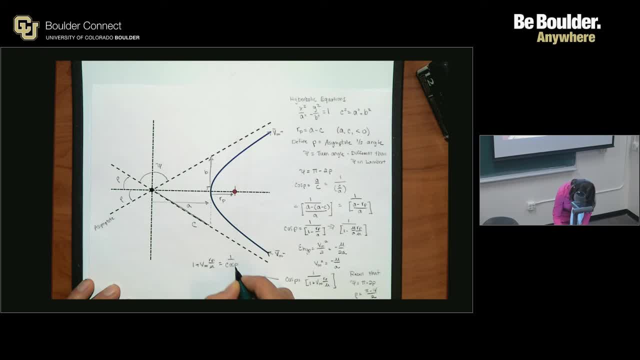 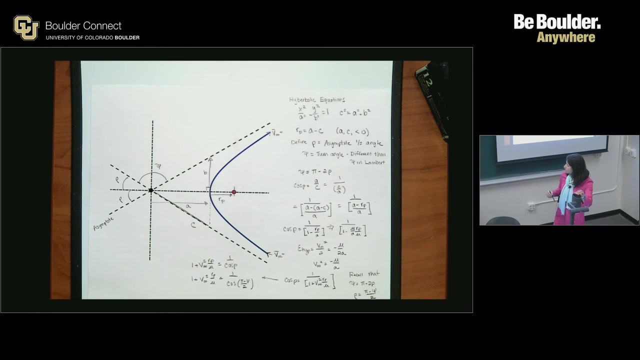 Yeah, Thank you, Yes, Yes. So one plus b infinity, squared r sub p over mu, is equal to one over the cosine of pi, minus psi over two. Okay, So we're getting really close to getting somewhere. No, That's as far out as I can go. 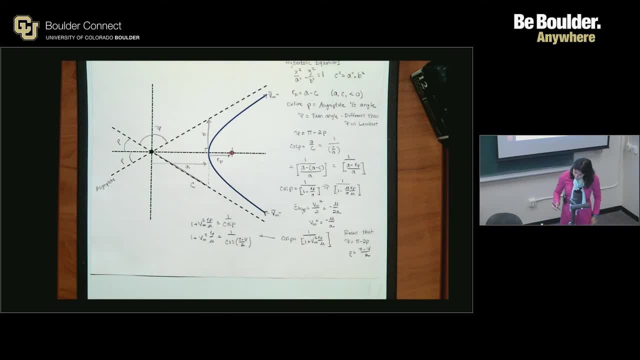 All right, I'm going to scoot this up. We can solve this for r sub p, because that's essentially what we're looking for. So we'll have r sub p. is mu over v? infinity, squared one over cosine of rho, All right. 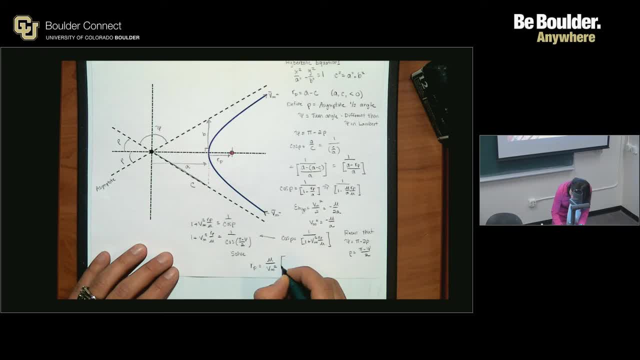 So we're going to solve this. We're going to solve this. We're going to solve this. All right, So we're going to solve this. We're going to solve this. So we're going to solve this. 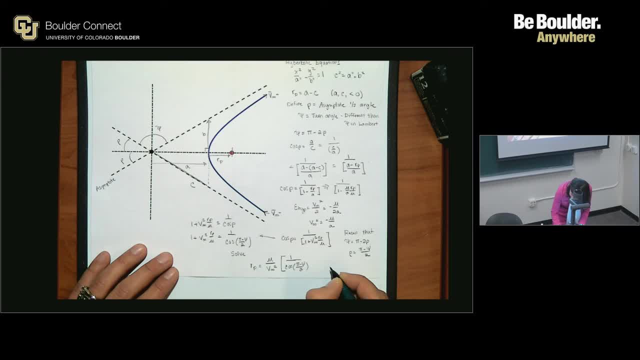 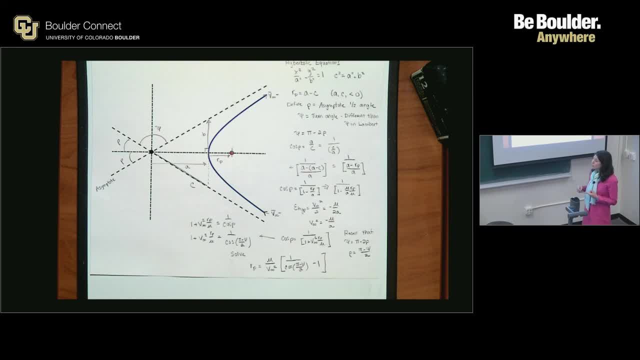 All right. So we've got this nice equation for r sub p. We know v infinity squared. What we need to find is psi. We don't know what psi is, but hopefully this will. we can show this real quickly. I'll just show an alternate view of a flyby. 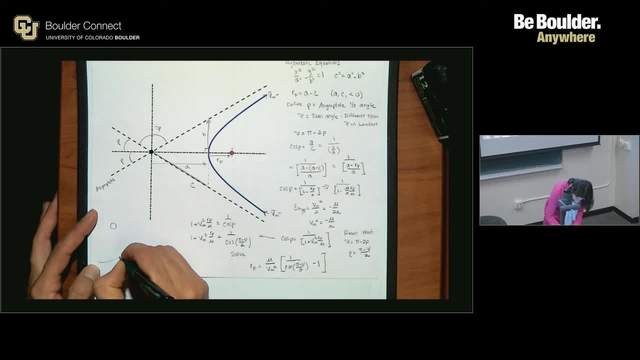 So if we've got a flyby that's doing something like this, Okay, So here's r sub p. You've got v infinity in and v infinity out. Here are the asymptotes. This is values of rho, and here's psi. 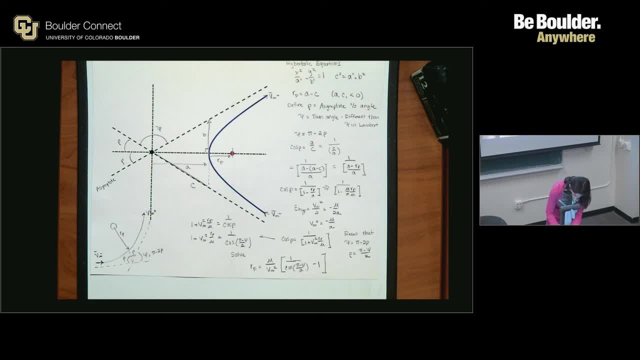 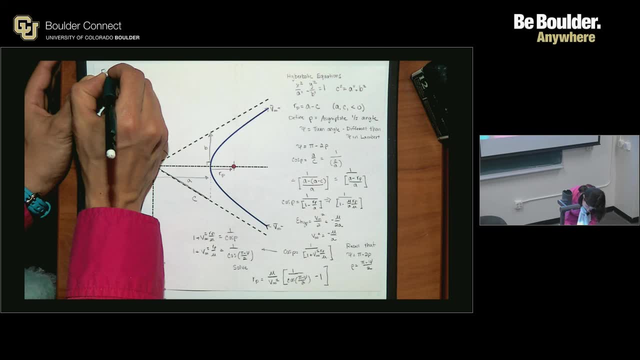 We can actually find psi from v infinity in and v infinity out. I'll do that up here. Sorry for the running out of room, So find. okay, we can do that Because we know the components of v infinity in and v infinity out.